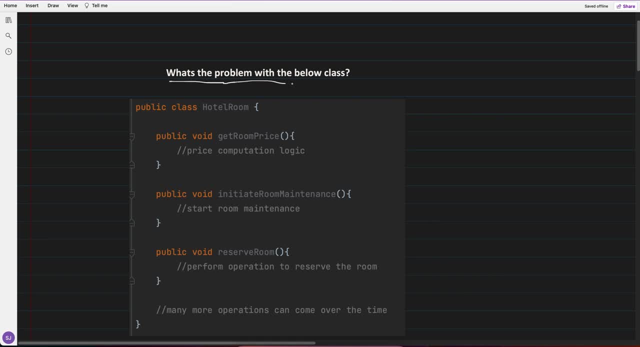 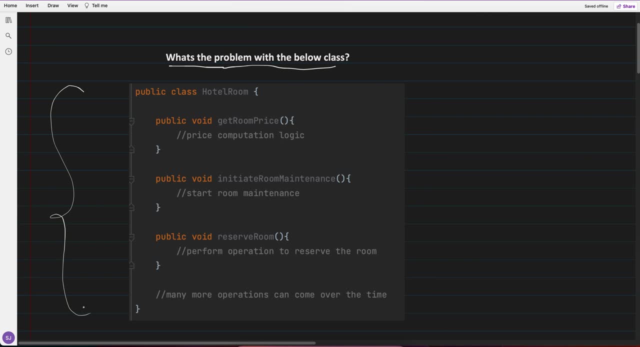 is: what is the problem? which visitor pattern solves actually? So can you look at this class and tell me, like, what is the problem, you see, with this class? Very simple class, right? So in my opinion, I can see that there are two issues with this class. One of the issue is that 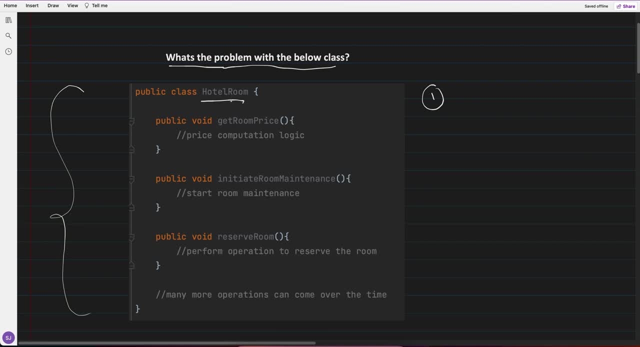 let's say this is a simple basic hotel room class right, And what I have added is operations. Okay, one of the operation is get room price. Another operation is initiate room maintenance. Third operation is reserve room. Similarly, more operations can overcome be added right over the time. 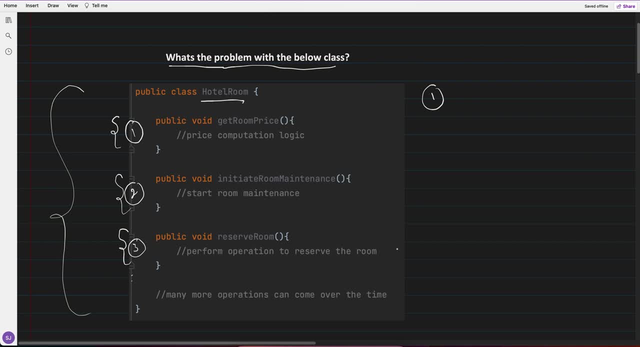 more operations can be added to it. So by looking at this class, one thing I know that okay, today, let's say with this three operations, I have tested my class fully, fully tested. But in future, if any new operation is added, let's say operation x is added, If any new operation 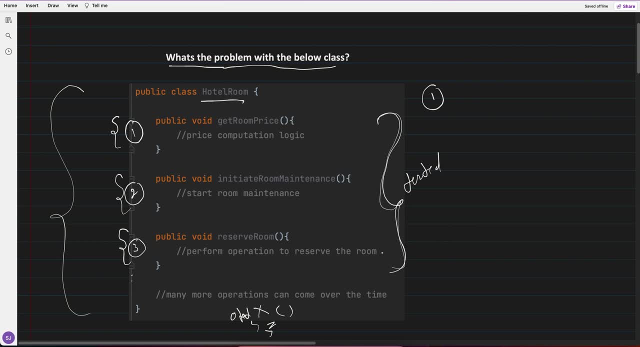 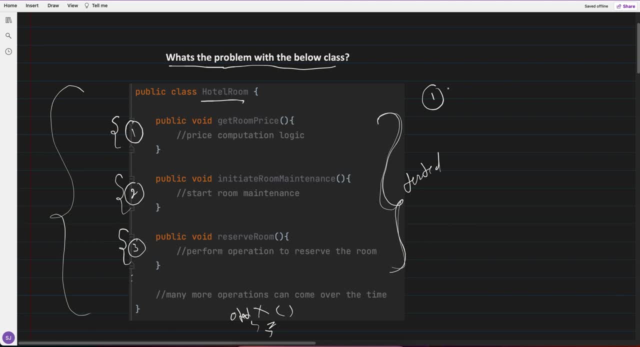 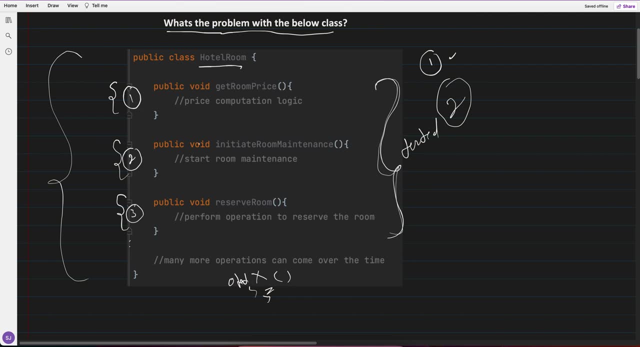 every time a new operation has been added to it. Right, So that is one of the issue. What is the second issue which I see is that this class can grow If you don't know how many operations can be added. let's say, slowly, today's only three operations. Maybe after six months. 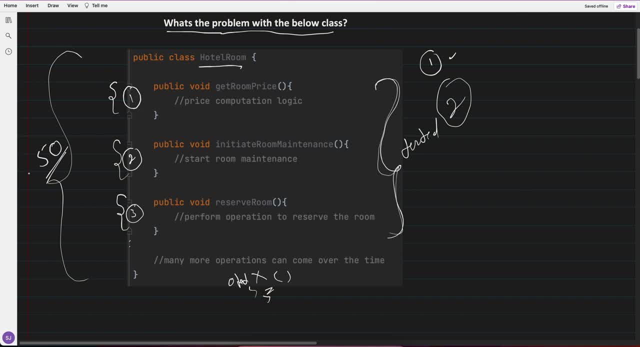 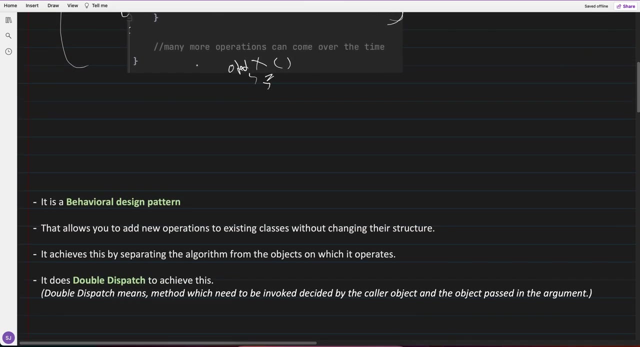 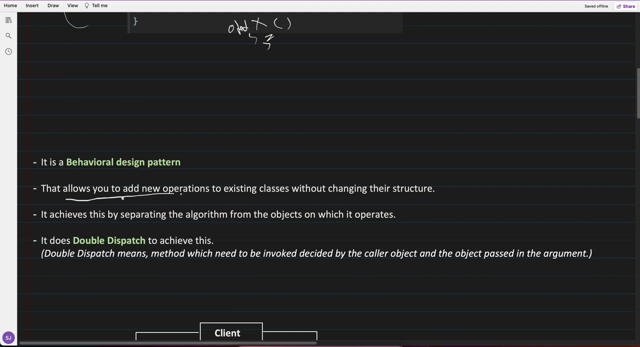 this class may host around 50 methods, or you can say that 50 operations, So this class can grow huge, Right? So that is a problem which actually visitor pattern solves, Right. And if you see the visitor pattern definition itself, what it says, that this pattern allow you to add new operation. 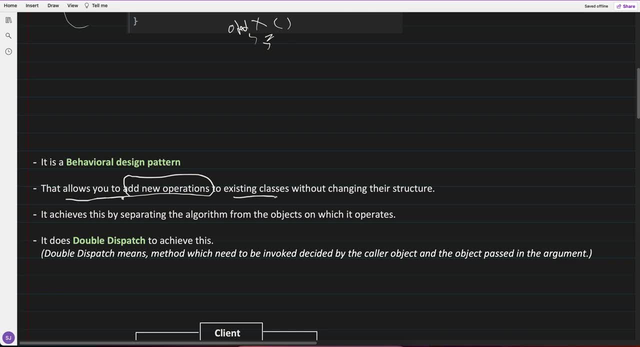 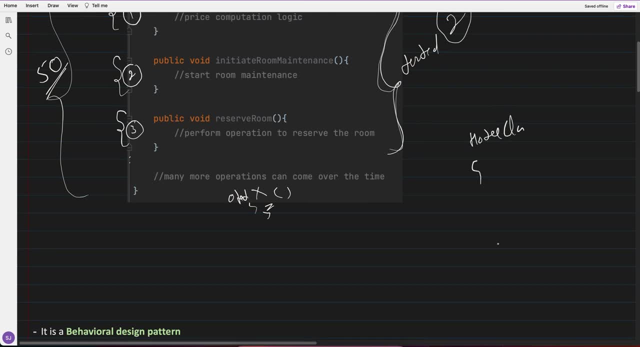 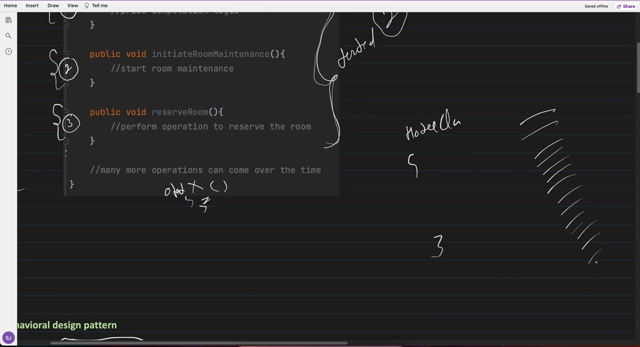 allow you to add new operation to existing class without changing their structure means to, let's say, that if you have created the hotel class today and you can add new operations, like in future, if, like, no matter 50 or 100,, whatever the operations. 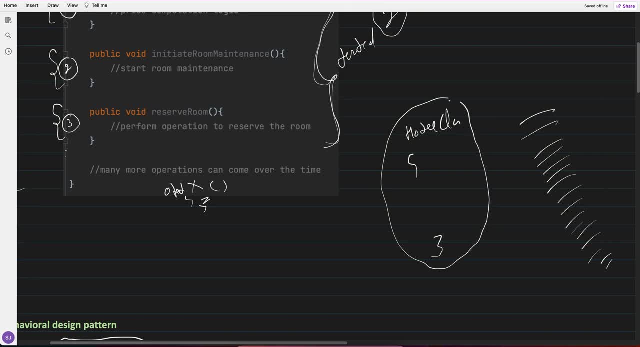 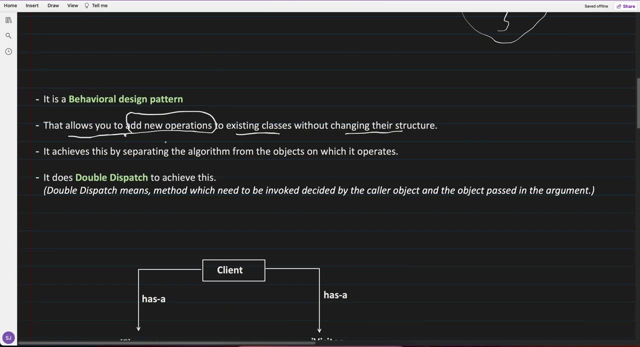 you are added, keep on adding it. you don't have to touch this. hotel class, hotel, hotel room class, Right. So that's the functionality. provide it. allow you to add new operation to existing class without changing their structure. It is achieved this by separating the. I would say that not. 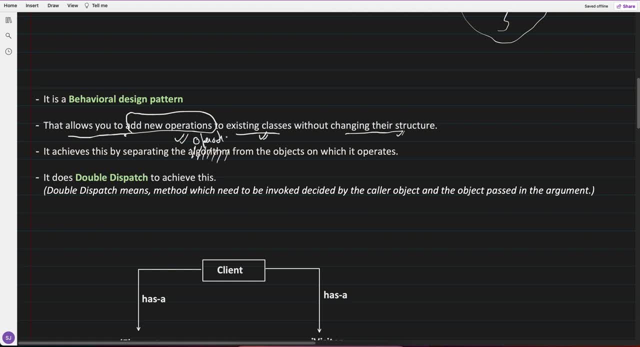 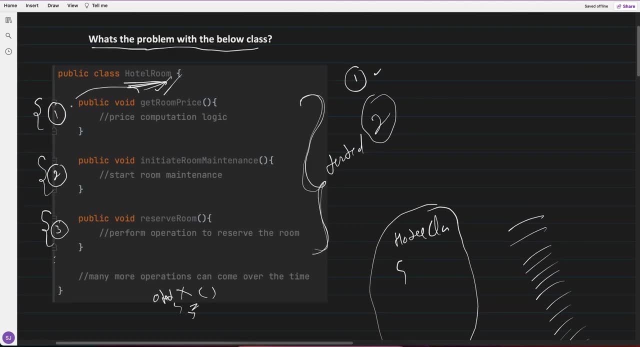 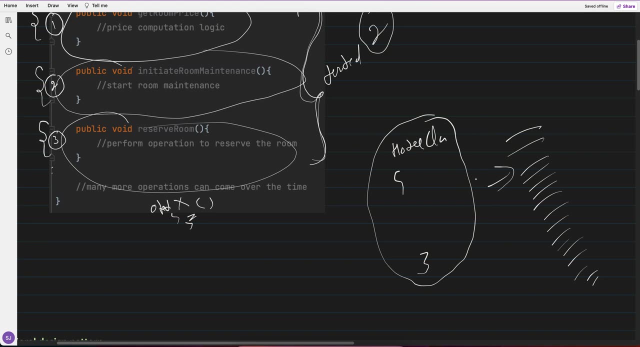 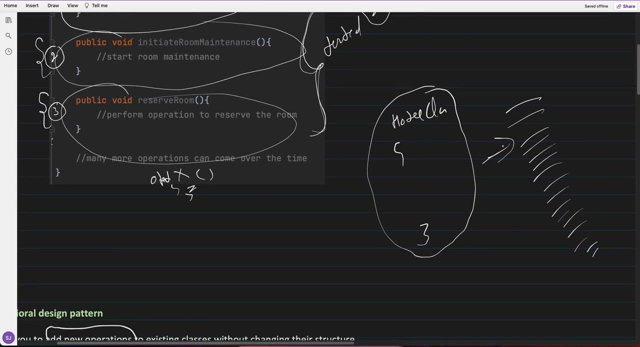 algorithm, I would say that separating the operation from the object on which it operates. So what it does is it takes all this operation and separate it out from the class. how it does how it separate out this operation. I'll tell you out this operation from the class and you can keep on adding on those operation and you don't. 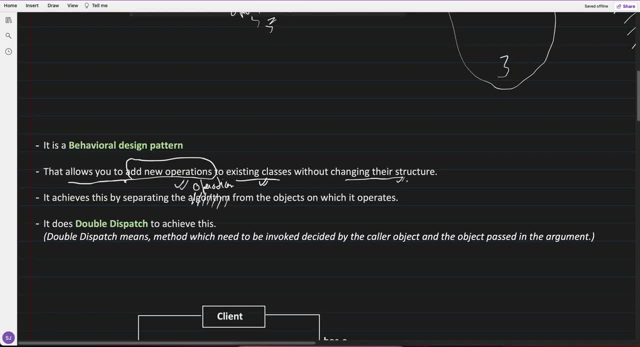 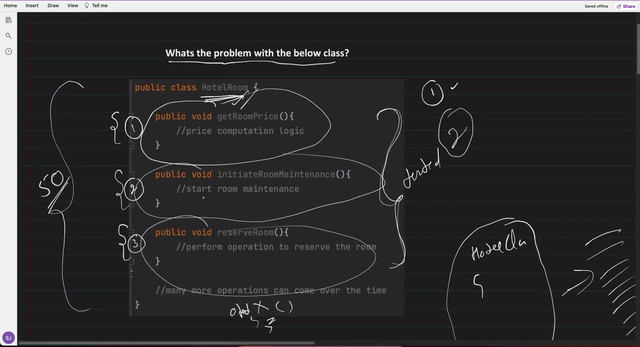 have to touch the class itself. Okay, so it is a behavioral design pattern, And you know now what it does. it allow you to add new operation to an existing class without you have to change it right, and it separate out the operation actually from the class, And this is the problem itself. 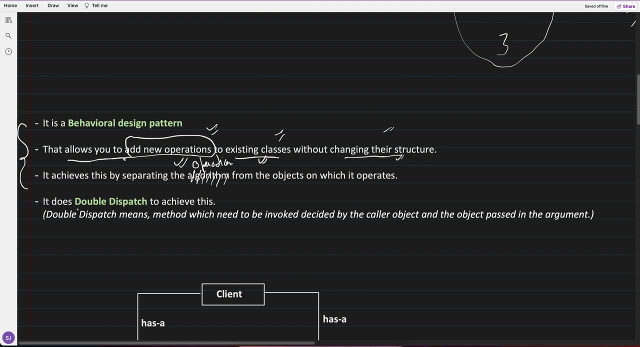 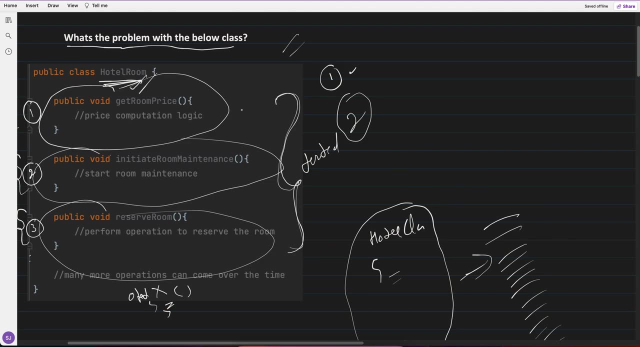 So by the end you will get to know about double dispatch. Actually, it uses double dispatch to separate out the operation from the class, When I was saying that, okay, from this class, we will take out all this, all this operation, we will take out from this class how it is, through the help of double 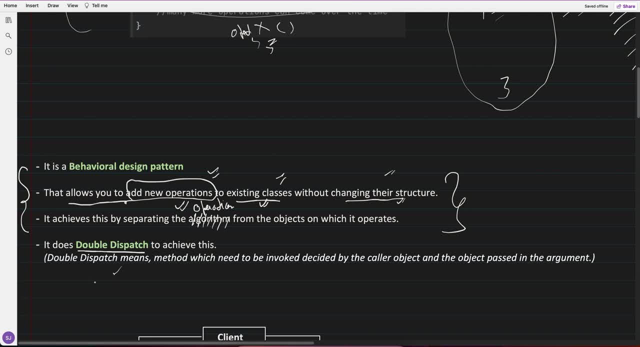 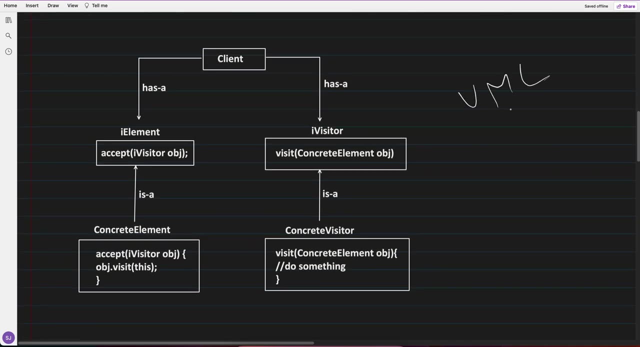 dispatch. So don't worry about double dispatch. Now, once we will understand with our example, you will easily get to know the. okay, this is what double dispatches. Okay, so we will come to this definition again. Let us understand with an example. okay, So this is a UML diagram. visitor design pattern- UML diagram. 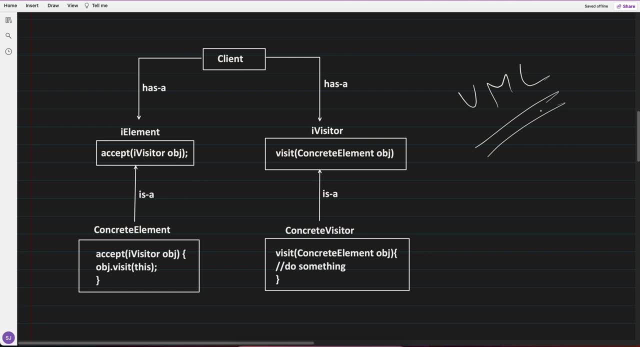 So here, very give, don't try to actually just give it a quick glance, then we will see with an example right, this UML become more and more clear. but at least have this terms in your mind that, okay, we have to create one interface. II tend for interface. 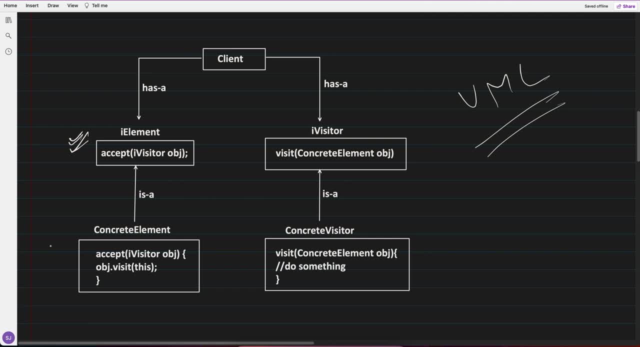 to create one element interface, then we can have so many concrete elements to it. so many concrete elements to it. similarly, we have to create one interface visitor. we can have so many visitor concrete classes of it. right, so two things: it has element and visitor. okay, so just have these two. 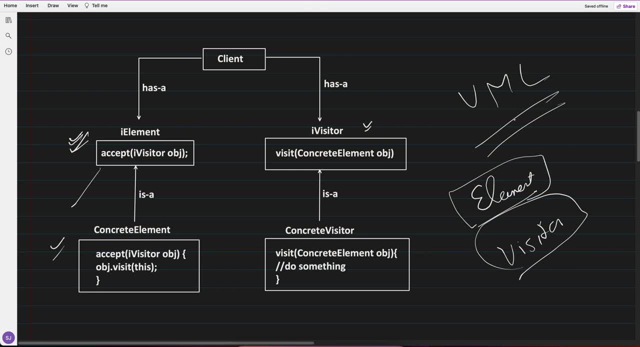 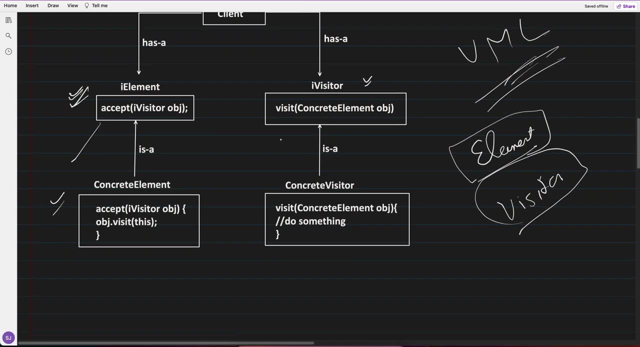 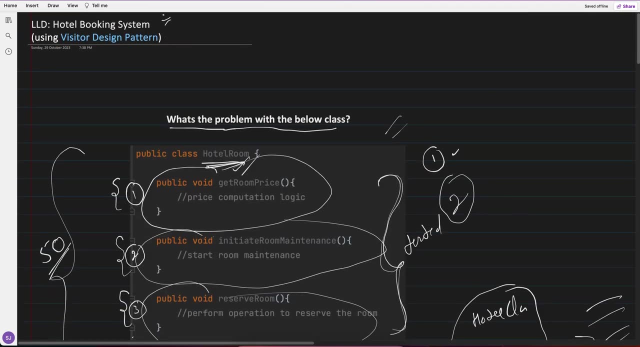 things. when we will see an example and then we will come back to this uml, you will actually understood this uml very, very properly, okay, so now i am taking an example of, let's say, a hotel booking system. let's say a very simple uh room, uh, room, tart. we will see. so let's see an example that. 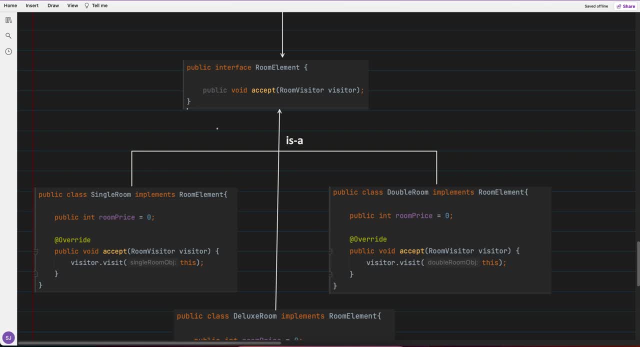 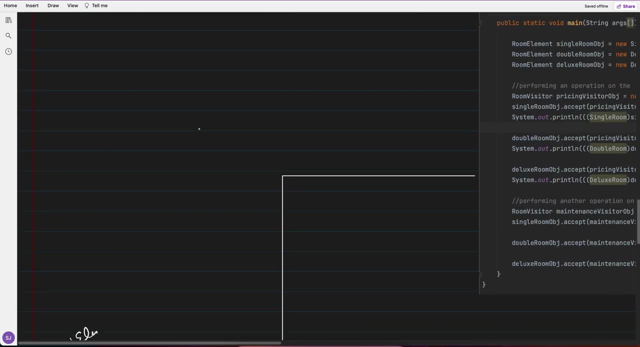 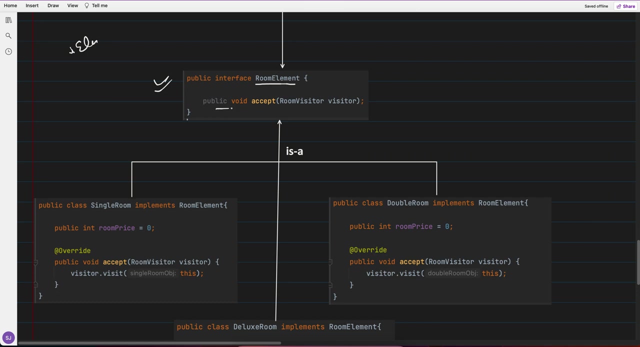 i am creating first this room element, interface, right, so this is your the i element which i created, right this part. so i am creating this i element. okay, so i created an interface room element and i have added one method except, right. so here, this except is what it is expecting. 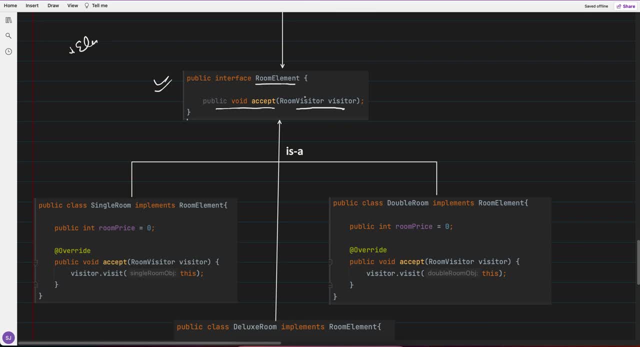 visitor element is our library, right? so this is the i element. okay, so we'll see that part. so here you need to first understand what is element. we are what, to whom we, to which object we are calling an element. so here you remember that i'll starting. i told you about hotel room. 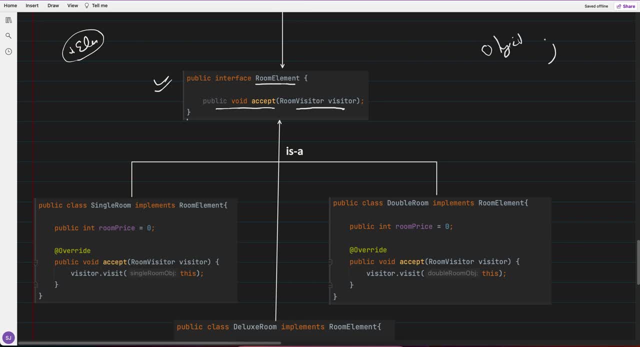 right, so that can be considered as an element. so any object on which you have to add operation right and you have to take out the operation out of this object, that object, we have to mark it as an element like. so from this element we will take out the operations. take out the operations from. 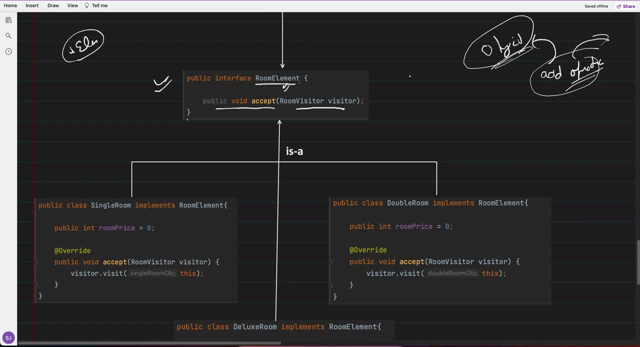 this element. okay, so from the above example, from the hotel room, we have to take out all the operations out of that class, right? so that's why i created that room as an element. so it's an interface and it is accepting one method. it has one method with the name accept. uh, we will see that. 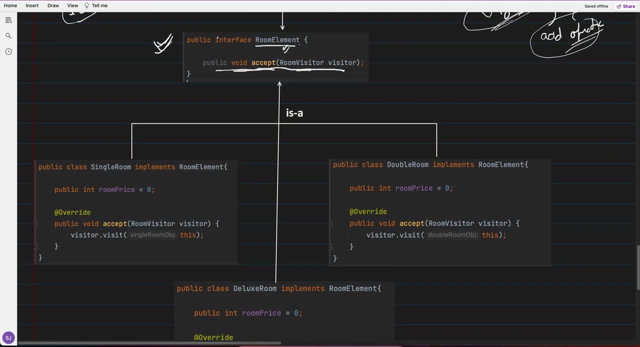 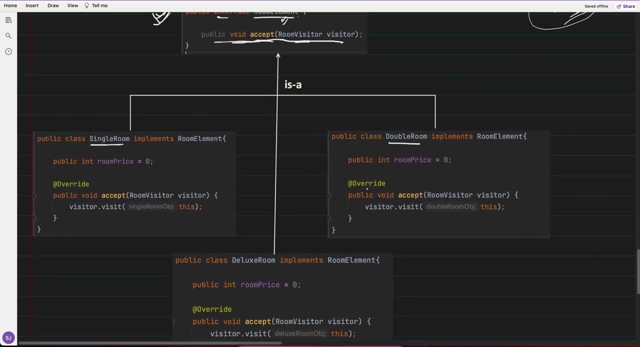 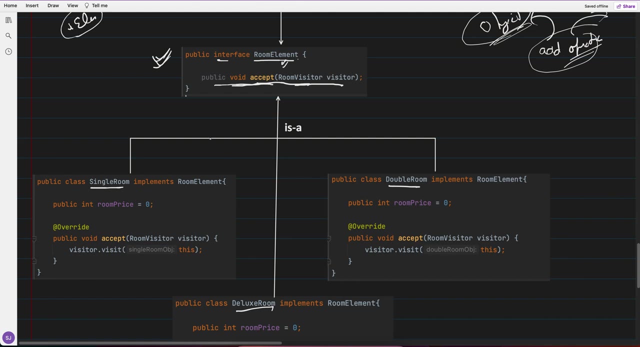 so now i created this interface right, there can be multiple type of rooms: single room, double room, deluxe room- right, so each are you can say that a child of room element. so they are is is the relationship right and they implements it. they implement themselves it: single room implements room element. double room implements room element. deluxe room implements. 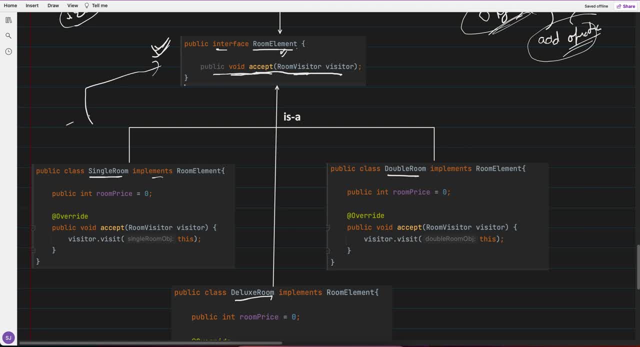 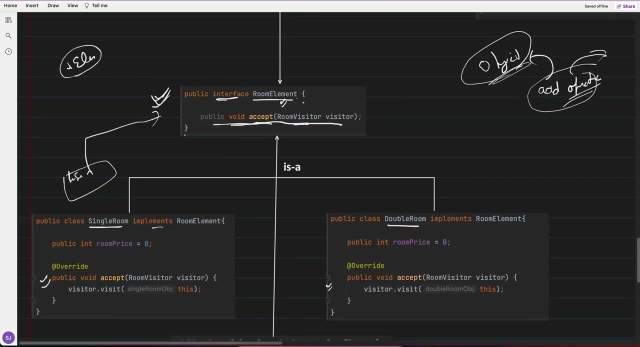 room element. in future maybe we can have another child class. let's say, a presidential suit implements room element, so they are different type of rooms in a hotel. okay, so since it's an interface, each child class has to implement this method. accept method: okay, so currently we are not seeing this accept method. we will see, like, okay, what this accept. 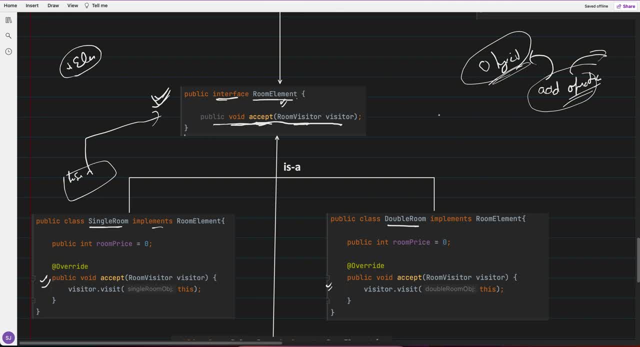 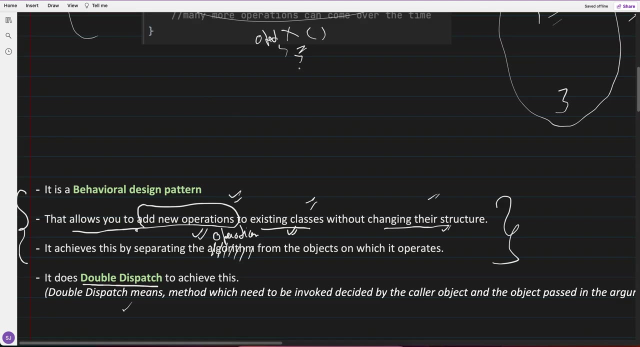 method does. but one thing: first point is clear- that to which object you have to create an element, the object from which you have to take out the operations right. so from rooms there can be multiple methods. we have seen right, multiple operations. i have to take out this operations. 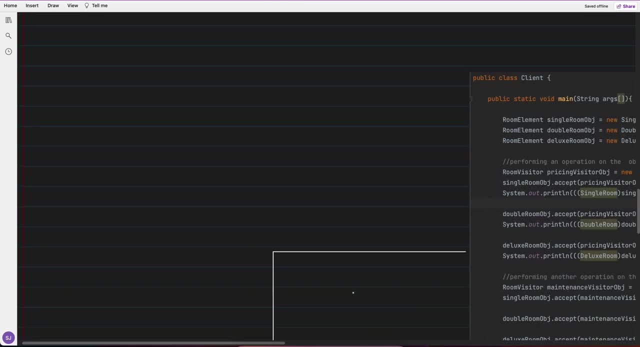 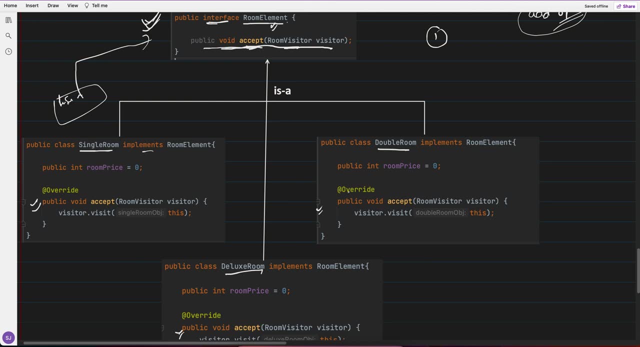 outside of this room. so that's why i created this room as an element and there can be multiple type of room: single room, deluxe room, double room. we can add those. it can grow in future also. now you can ask me where are the operations and where are those, how we are handling this now. room reserve room. 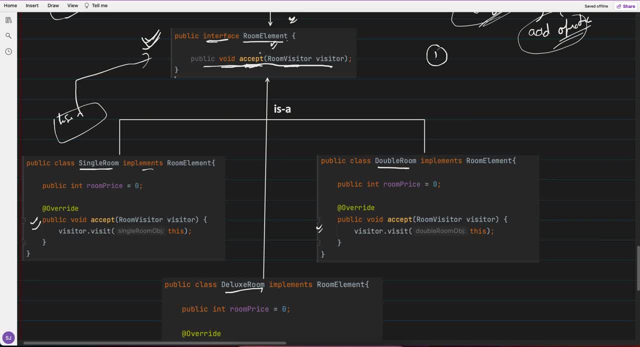 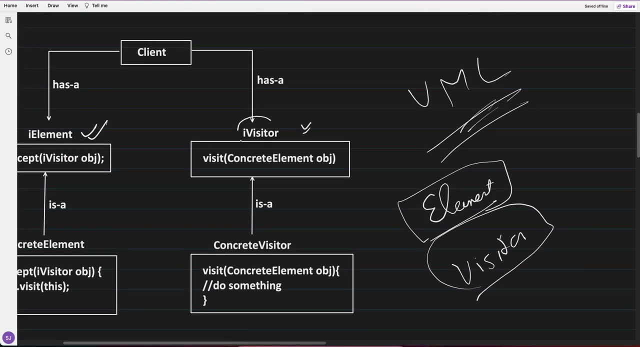 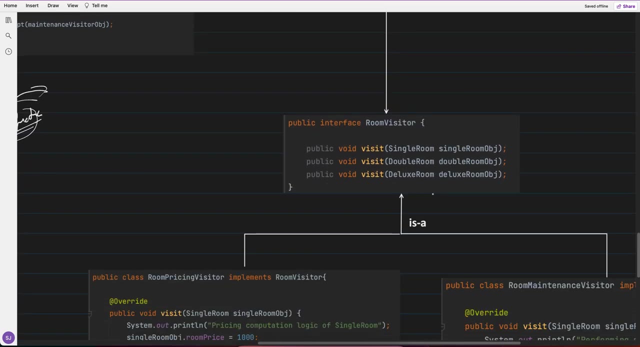 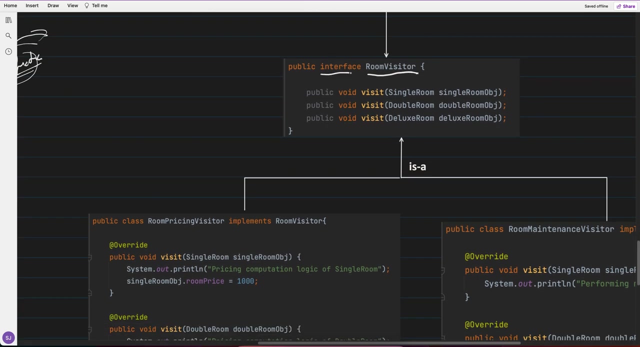 room price, how we are adding it. it has just one method. except now here, if you see that the second part comes is in our uml, is visitor right. so visitor is something which host all the operations. so now here, if you see that i created the room visitor right in this room. so this is an interface. 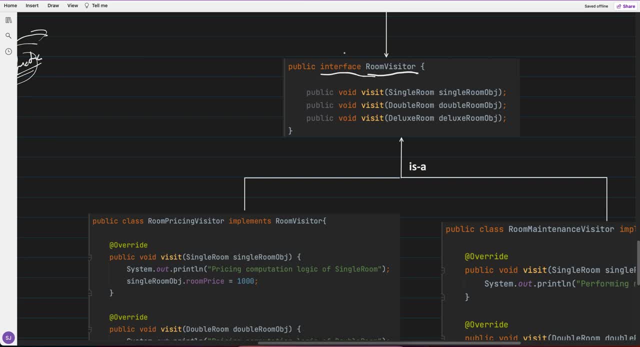 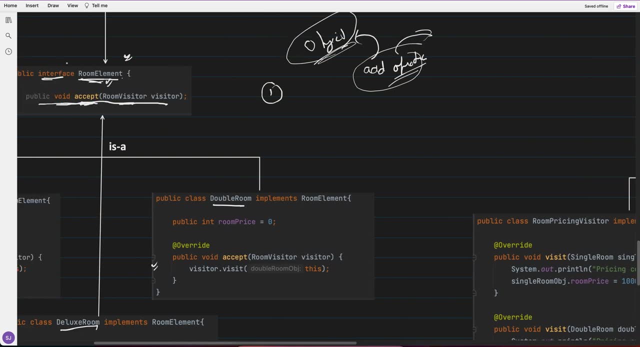 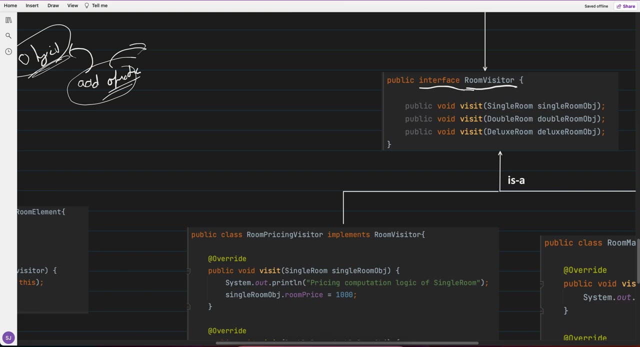 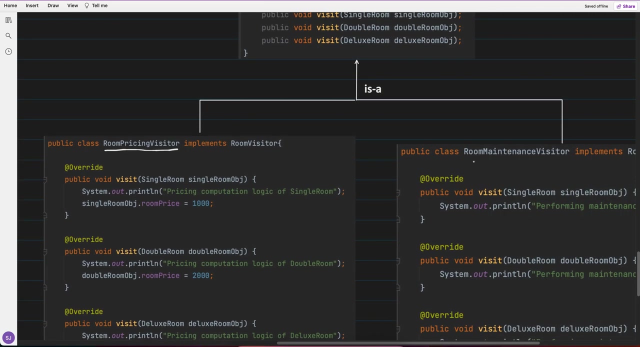 now all the different type of operations that can be done on an object. so my object is room. so all the different type of operations that can be done on a room. we can have concrete classes for it. so let's say, for room visitor, i can have room pricing visitor. another is room maintenance visitor- you can add more. 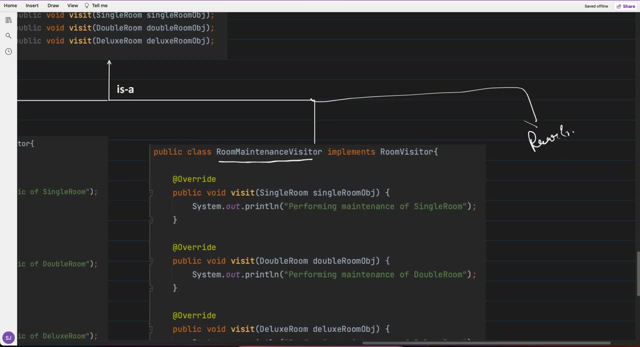 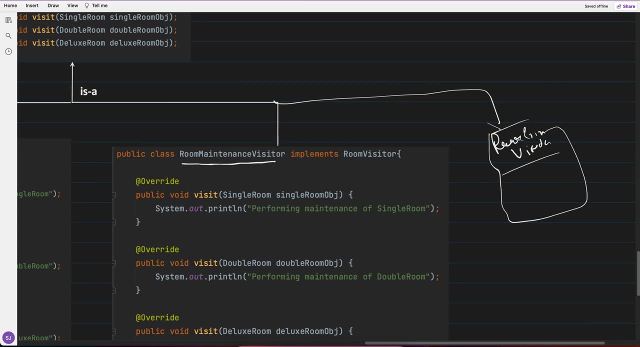 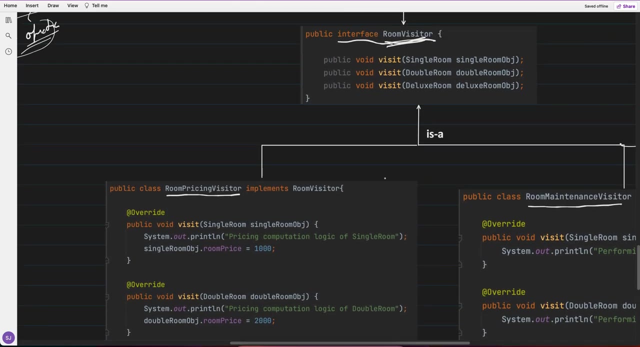 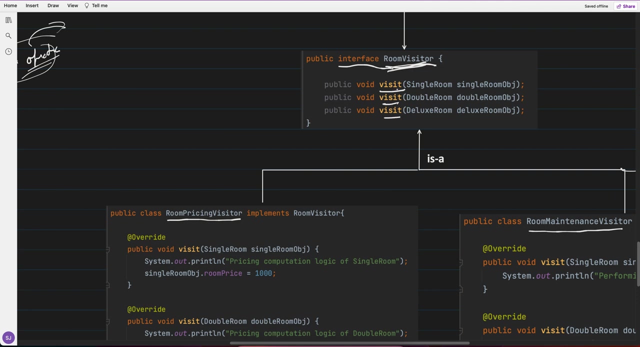 what are the different operation? reserve room, reserve room, visitor right, so you can have. for each operation you can create visitor. you can create visitor now here. if you see that in the interface what method we have is visit right and if you see that we have one method for each. 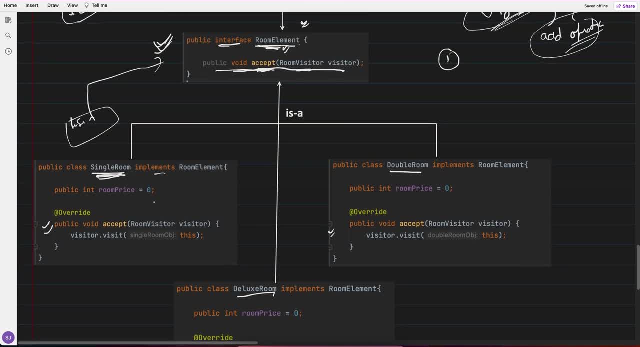 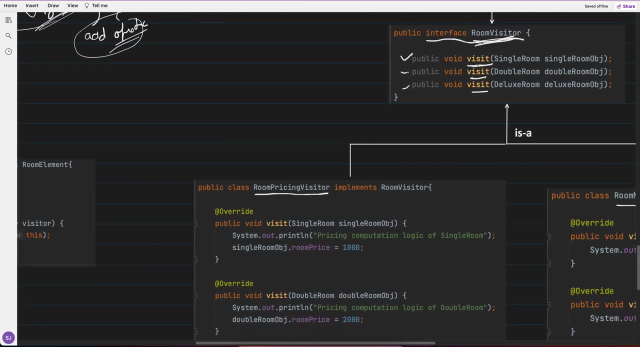 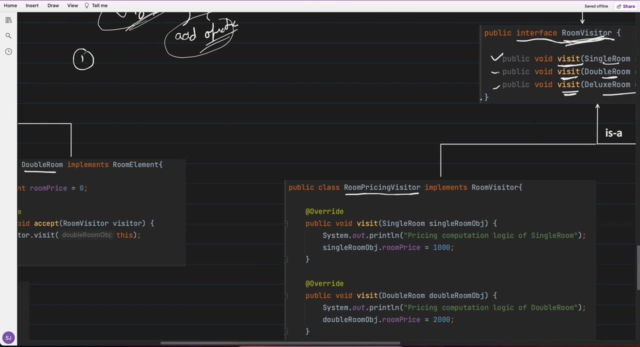 of this concrete element for each of this concrete element. okay, so here, if you see that i have one visit method which accepts single room, i have visit method which accept double room. i have visit method which accept deluxe room, right, which accept this object. now i should be able to perform. 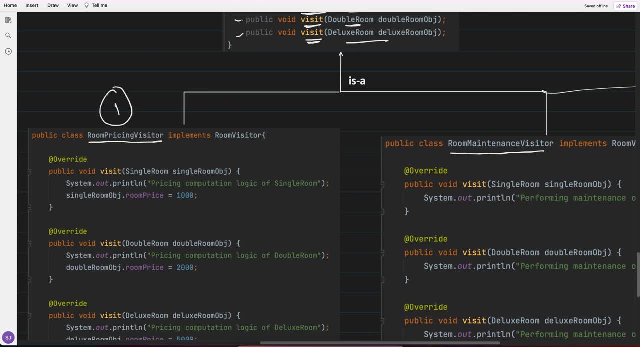 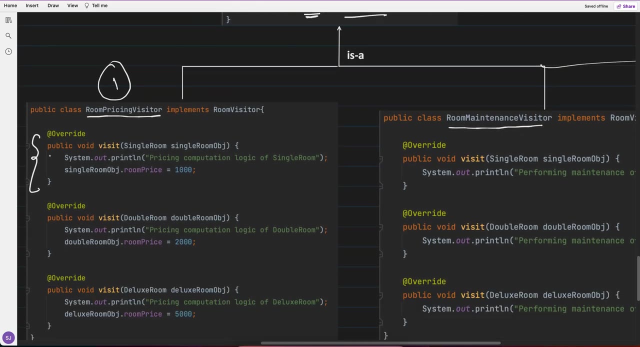 multiple operations, right. so first operation: i have created a concrete visitor class room pricing visitor. so here, if you see that i have implemented this method, visit method for a single room, i have added my logic to compute the price, so it is pricing visitor, right, so pricing related. 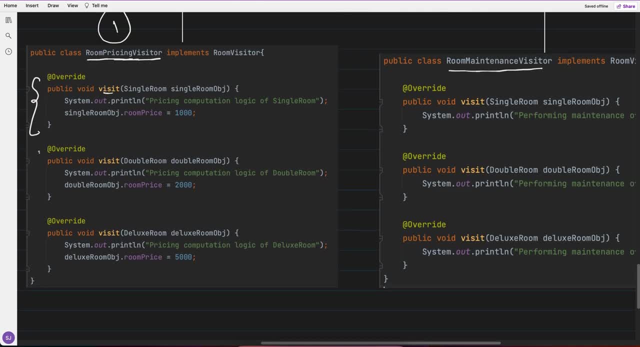 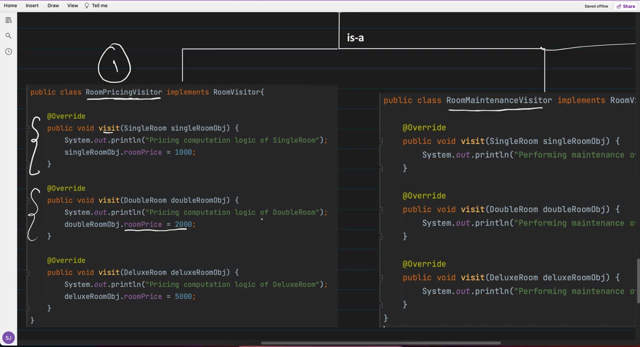 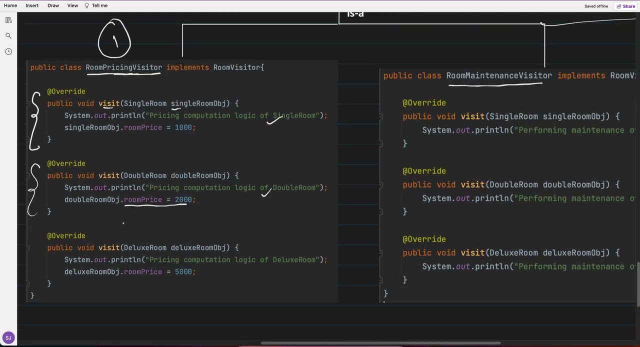 logic i have put into this visit method. then for double room. double room has its own pricing logic, so it is setting its own price price computation logic of double room. so in the single room, price computation of single room. third method is for deluxe room. right, so here i can have operation for 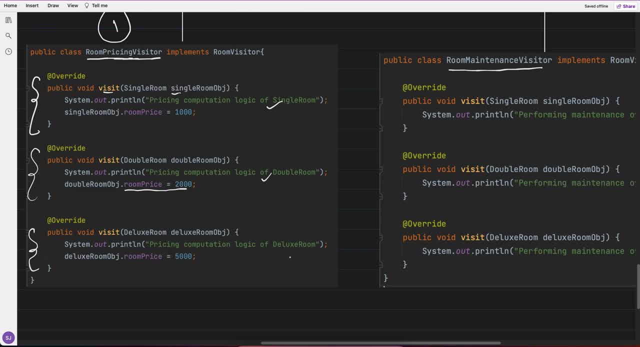 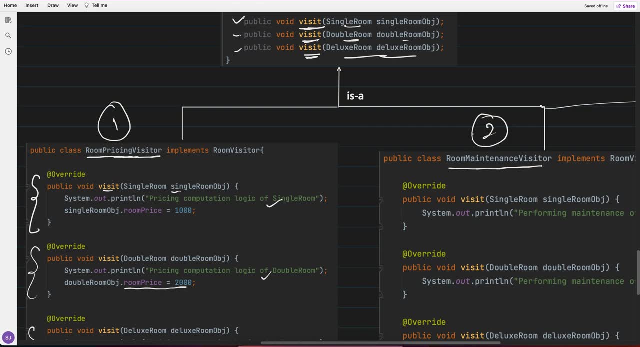 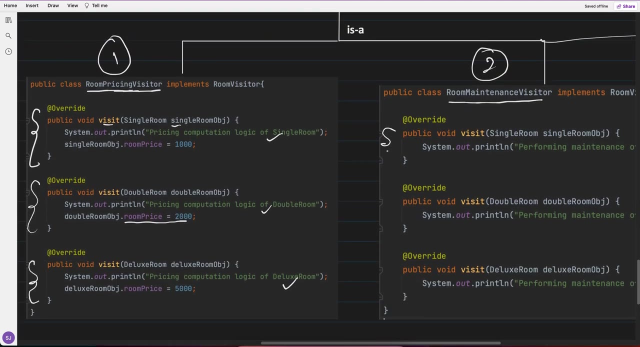 a pricing for this room, pricing, computation logic of deluxe room, so we can have that right. second operation which we wanted like say on this room is maintenance right. so for each method now if you see its implementation, they are doing kind of a maintenance work. so for the single room, it is performing maintenance of single. 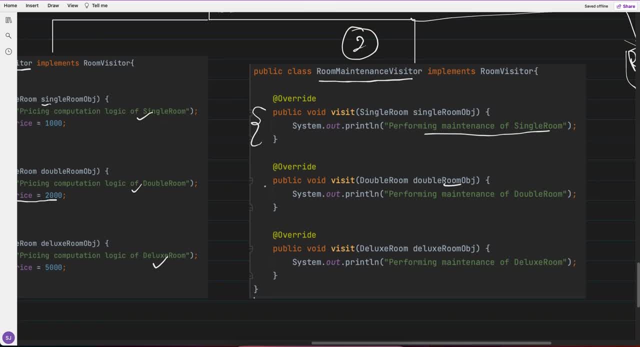 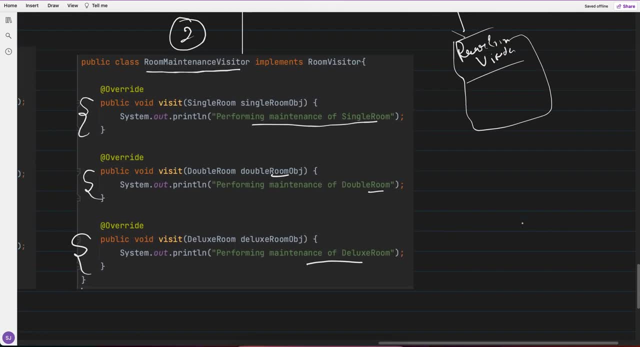 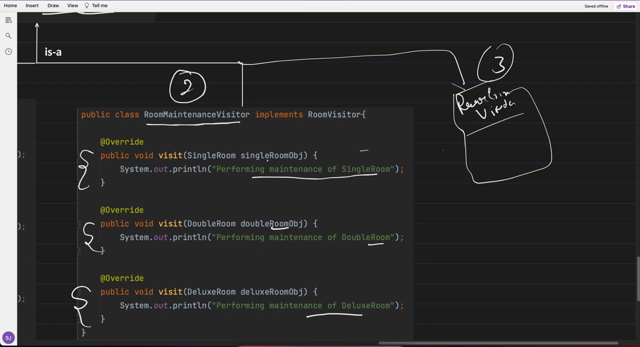 room might be some other logic for double room method. it is performing a maintenance of double room for deluxe room. it is performing a maintenance of deluxe room. it is performing a maintenance of deluxe room similarly. third operation: reserve room. so we can have all these three methods and they perform their own operation on the particular objects. so now, if you see that, what? 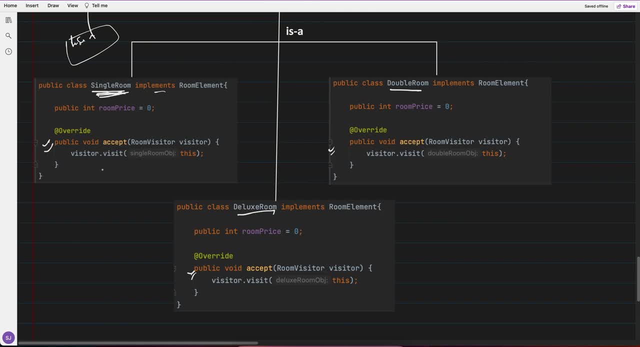 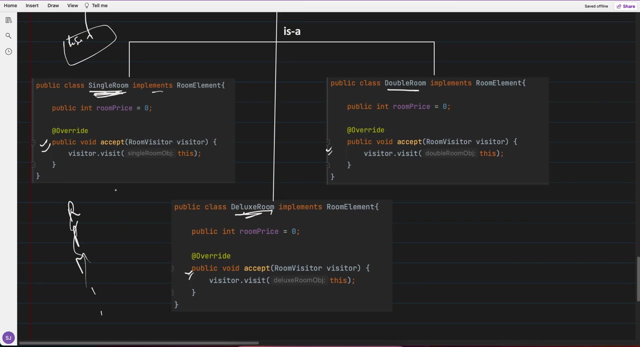 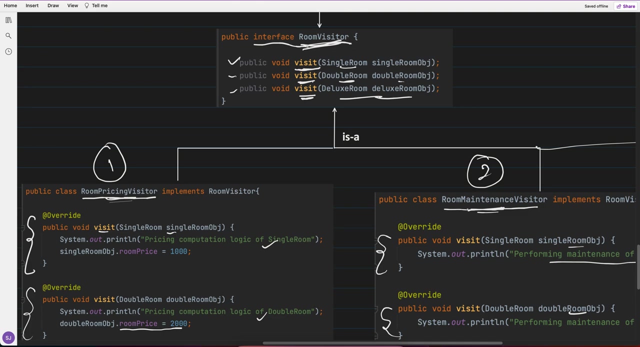 we have done is: single room might have multiple methods, deluxe room might have multiple methods, like reserve room, price maintenance and more. now here, if you see that those methods are not present here, those methods are gone there, visitor. so we have created a for each operation. we have created a. 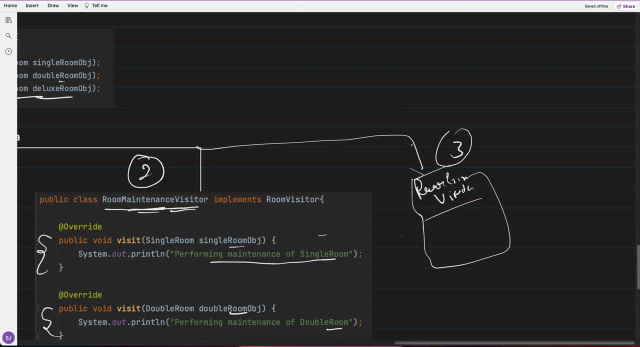 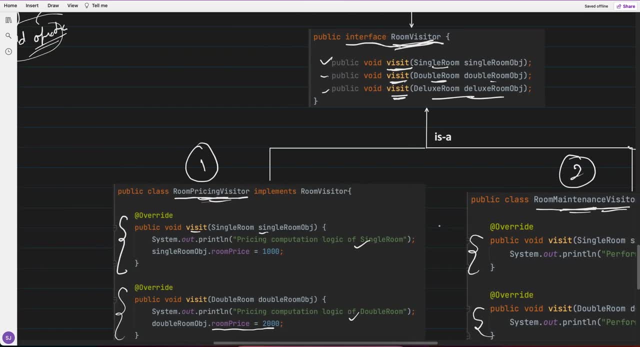 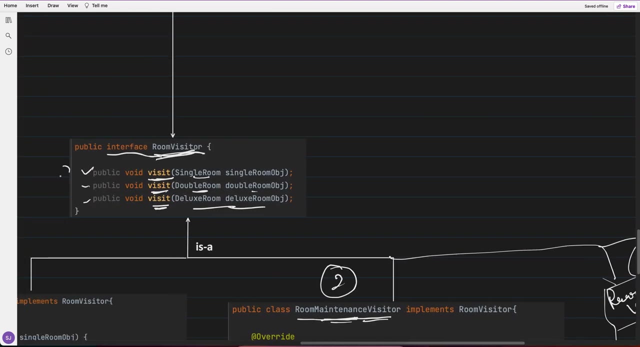 visitor right. so maybe in future we have any new operations coming in, we can just add a new visitor right and for all this elements, we will support these methods. right, for all this element, we will support this operation. let's say, in future we will add a new method called presidential suit. 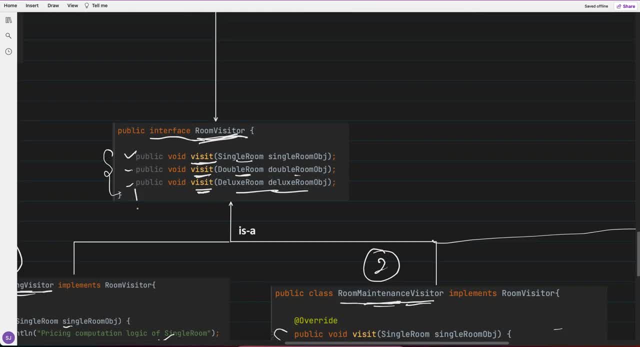 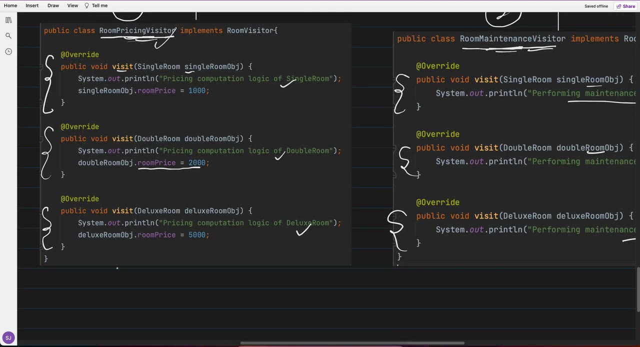 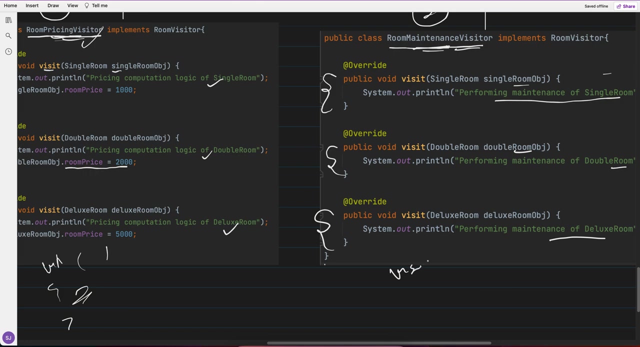 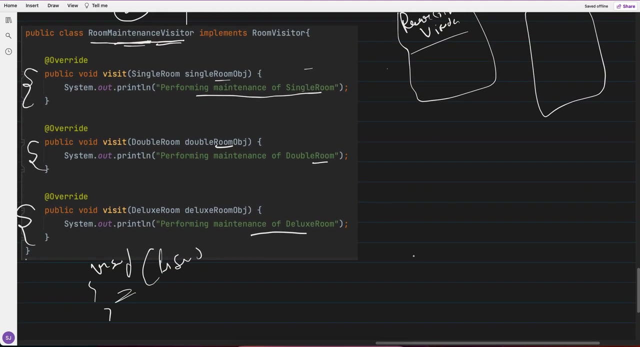 new element, presidential suit, so we have to add it here: public void, visit presidential uh uh, presidential suit and its object right and we have to provide its pricing, its pricing here. we have to provide its implementation maintenance. we have to provide it uh implementation, visit presidential suit and provide its implementation for reserve. we have to provide uh implement this. 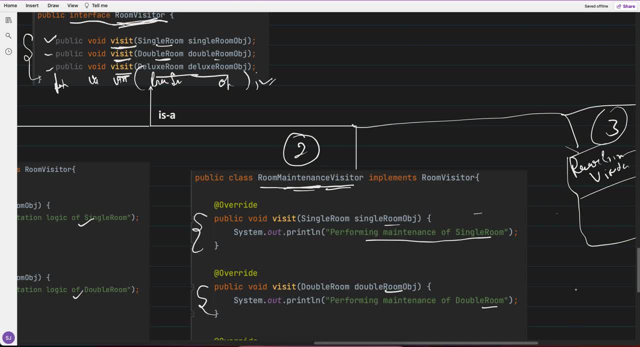 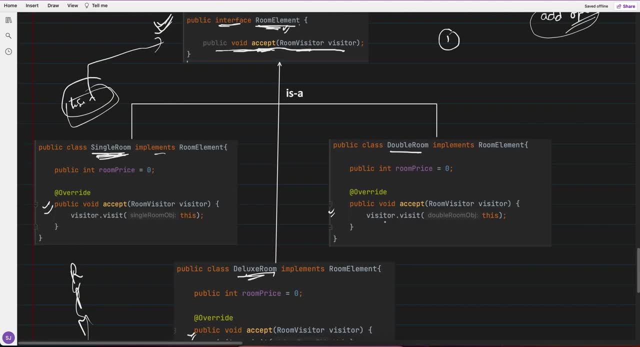 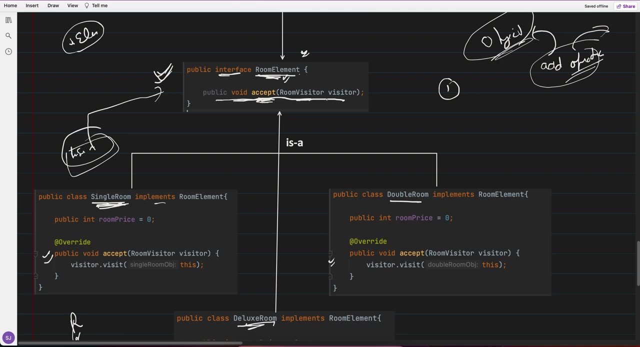 method and provide that implementation right now, here. if you see that how it is working is so now. now look at this method again. accept method which is presented to the element. so here it. accept a visitor, like: what visitor you want to pass? if you are passing a, uh, uh, a visitor, you want to pass a. 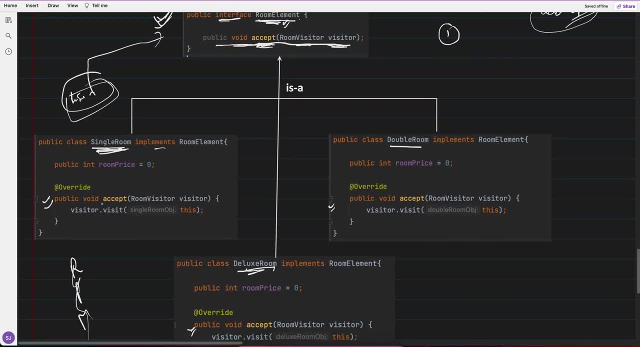 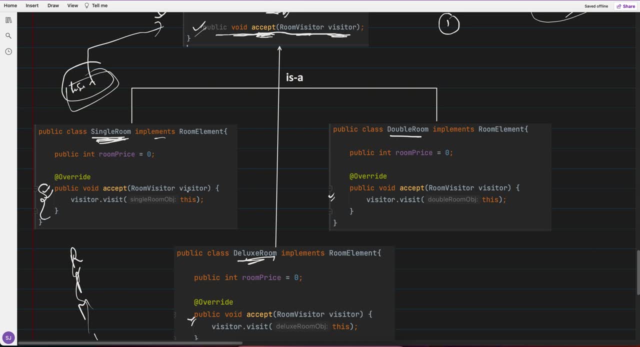 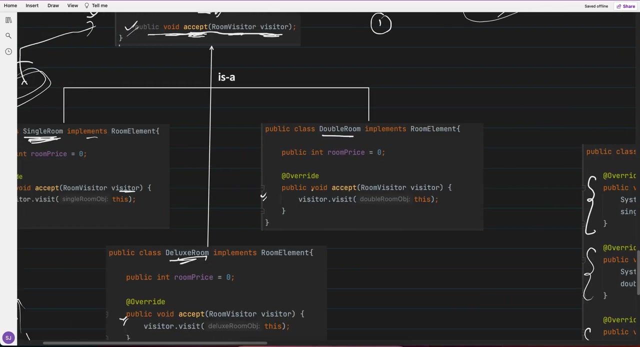 a room pricing visitor. and here, if you see that this single room implementing this except right. so here let's say: visitor, i pass, i want to calculate the price right. so from the uh run time the client can pass the visitor of this one, this operation visitor, room pricing visitor, then it will cause. 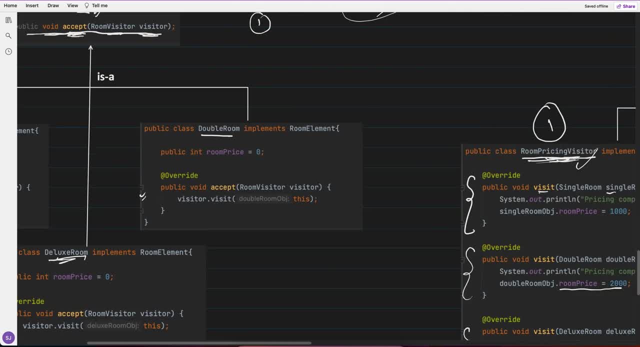 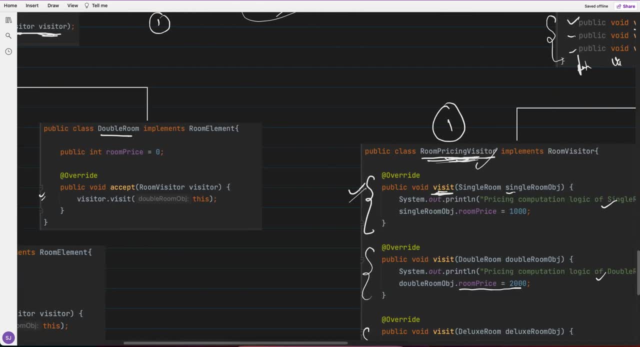 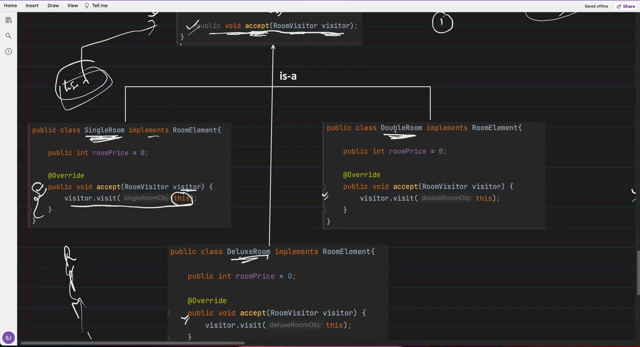 its visit method. it will call this visit method. right, which one from single room? right, i am passing single room, object this. so it will call this method. let's say, for uh, double room, you want to invoke the maintenance or method, how you will uh initiate the maintenance method? so here, if you see that, 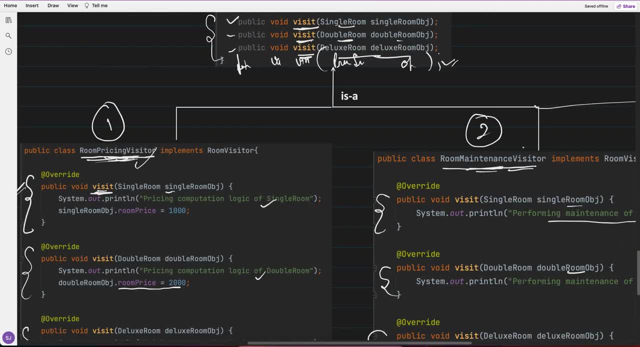 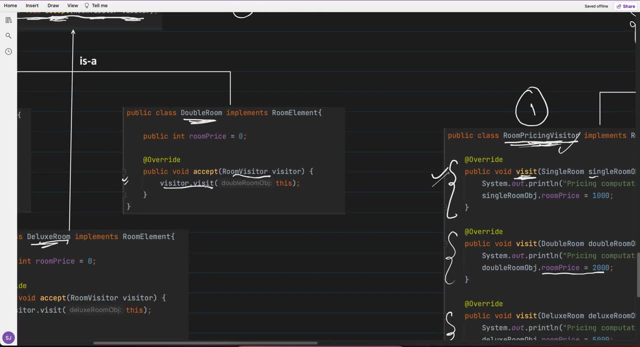 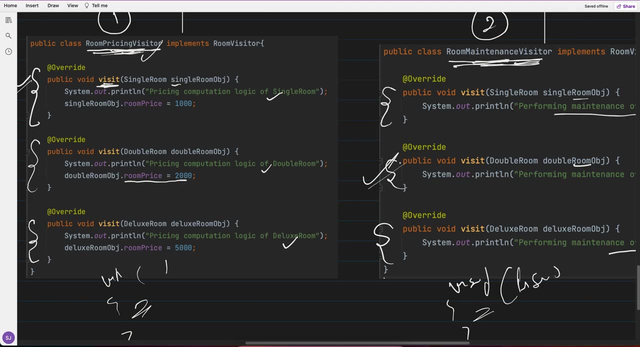 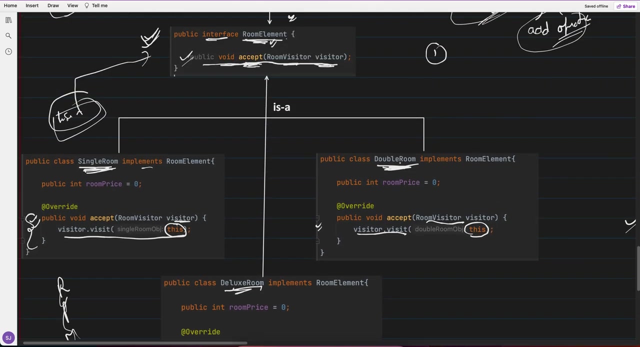 in the room visitor i can pass an object of this visitor, room maintenance visitor. and room maintenance visitor will call the method visit. now which method to invoke this double room object? so it will call this double room maintenance method, right. so both the problems are solved with this right. so first problem is that let's say you have 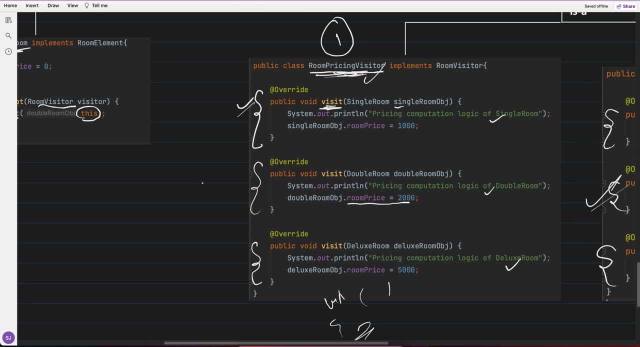 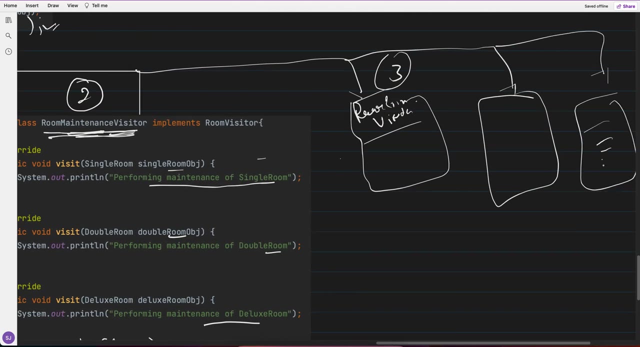 tested this class. you have tested this class. you have tested this class. room pricing visitor. all the operations are tested properly. right now. let's say you are adding new operation. you are adding new operation. you are adding new operation right, a reserve room. do you have to touch this room? maintenance visitor. 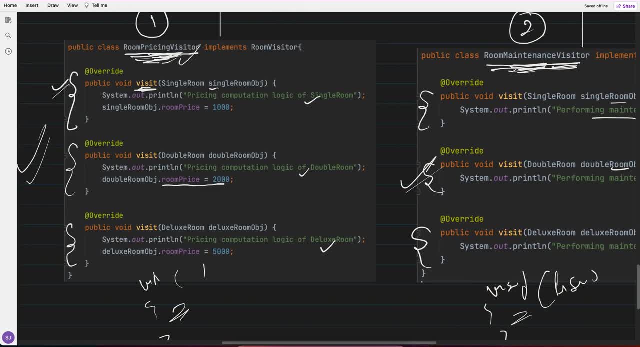 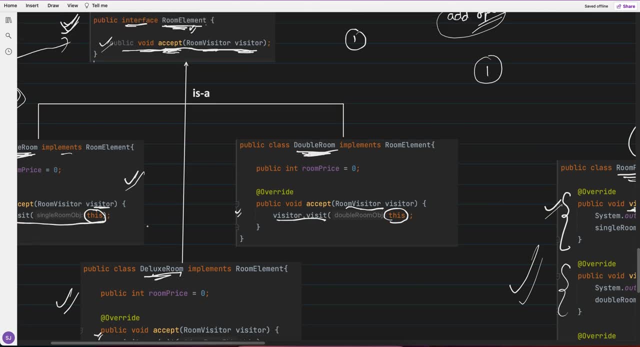 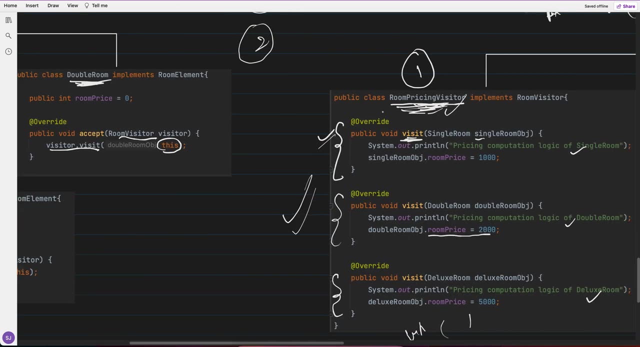 method? no, do you have to touch this pricing visitor methods? no, okay, so once you have tested any new operations added, you won't have to touch it. second thing is: will a one particular class will grow? no, so here, if you see that, this all, so, any new operation will come, it will grow horizontally. 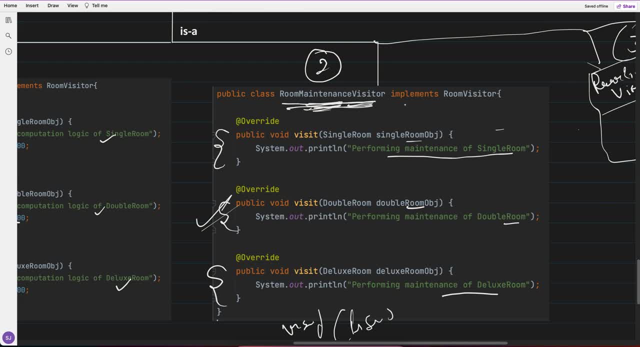 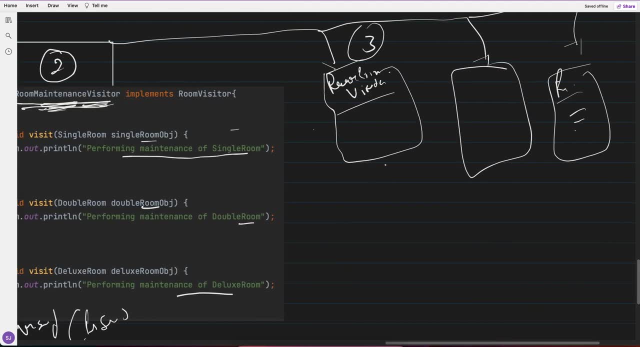 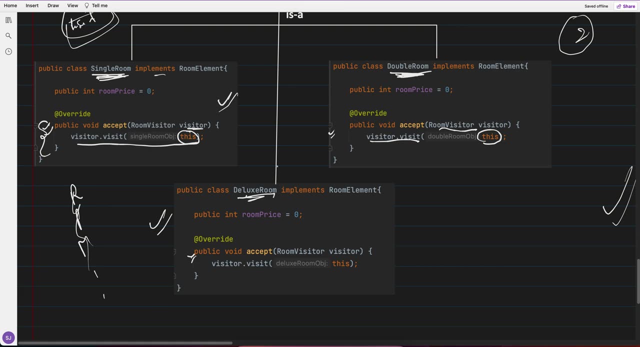 not vertically. one class will not grow to a massive, it will grow like a horizontally. for each operation we will create one visitor right and it can grow horizontally right, and they support a method for each of these elements. now, here you can ask me right, hey, shams. 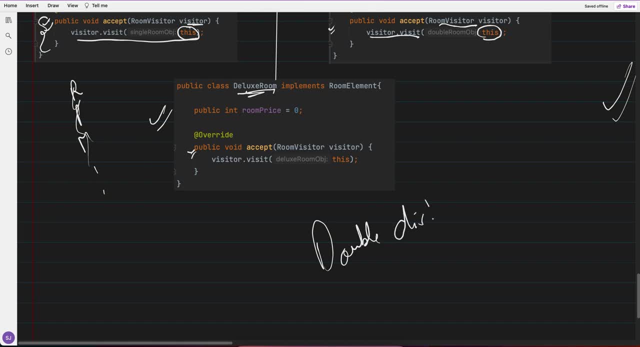 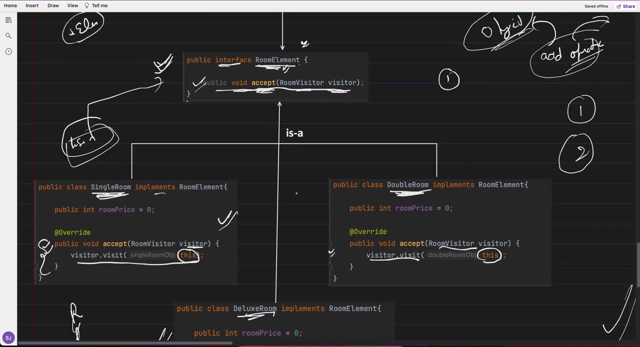 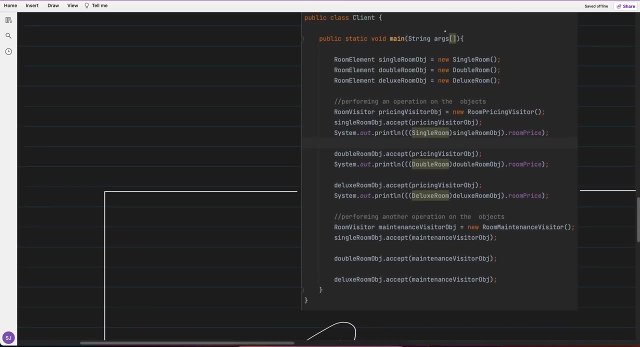 how the partАnyou going okay, so tell now. you understand here, right, what we are doing. so here now, let's say that we have to call whatever this is. let's say: this is the method. now i have created an object of object, deluxe room object. so i am creating three objects here now i am performing an. 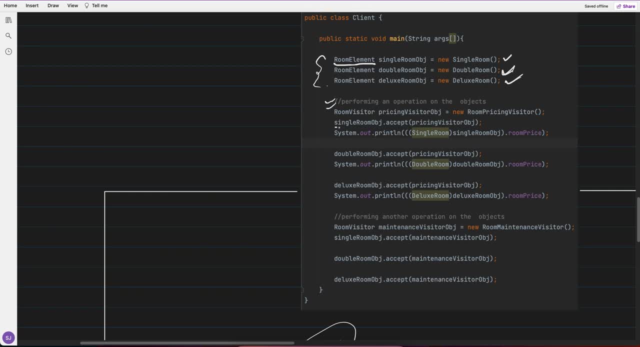 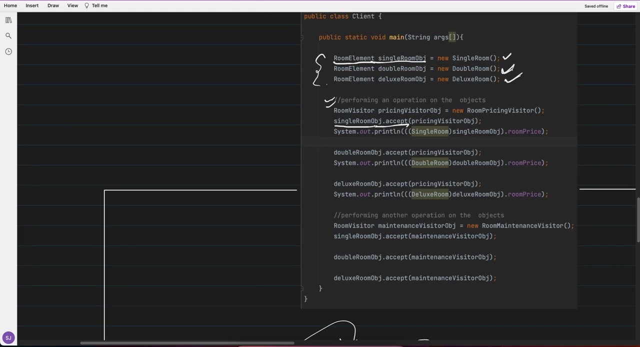 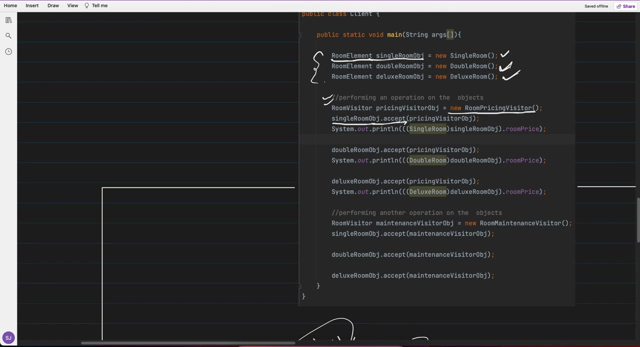 operation on the object right. so first for the single room for this object i am calling the except method, but i wanted to call a which method, pricing method. so i am which visitor, i am passing it. room pricing, visitor method. object right. so when it called the except, 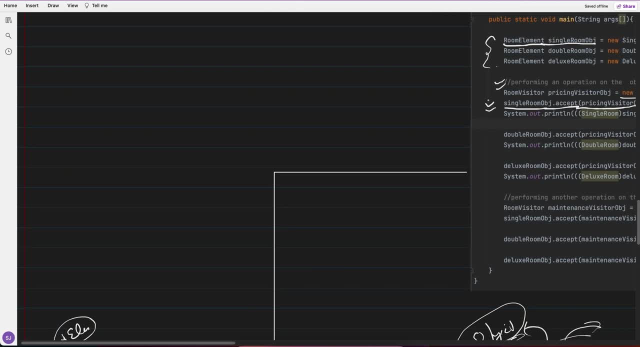 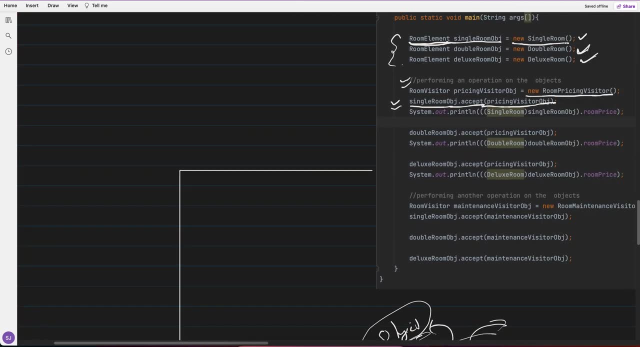 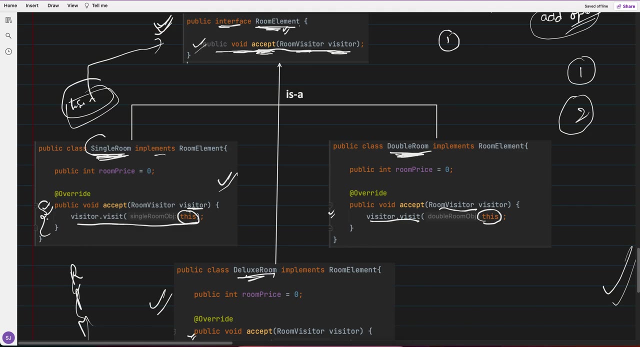 single room object: dot except. so single room object is a room element, it's an interface, but the object it has is new single room. so it which except it will call invoke. it will call invoke of single room. this except will get invoke. this will get invoke. ok, now it. 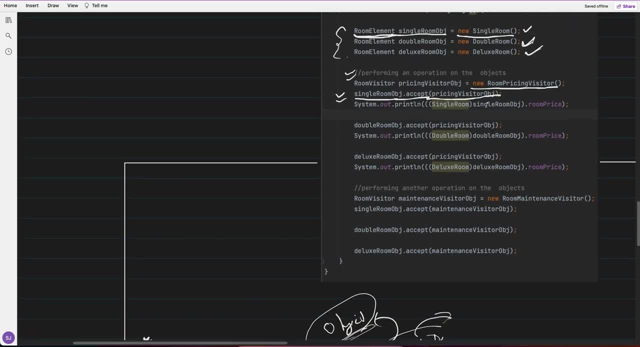 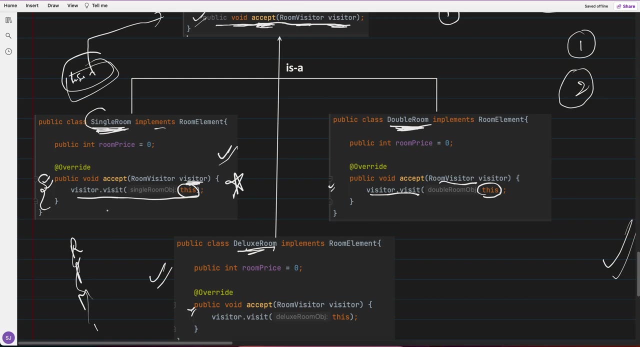 invoke, and in the argument, what object we have passed? we have passed pricing visitor, object this one. So again, this is an interface, But what object it holds? room pricing visitor. so now this room pricing visitor, here i am calling the visit method. so in the room pricing visitor it is calling the visit method, which. 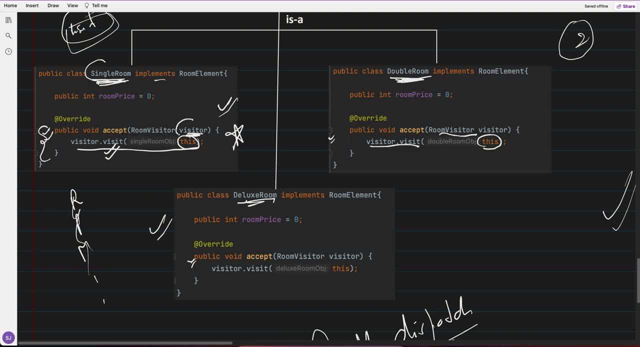 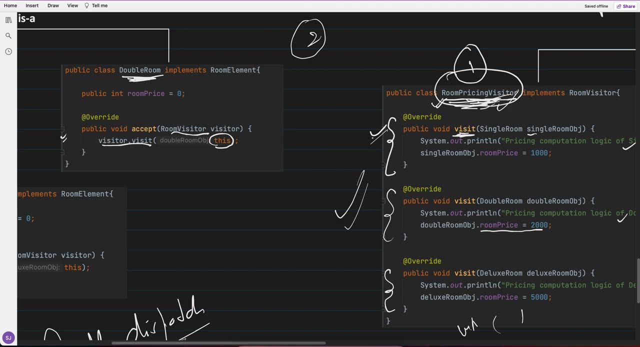 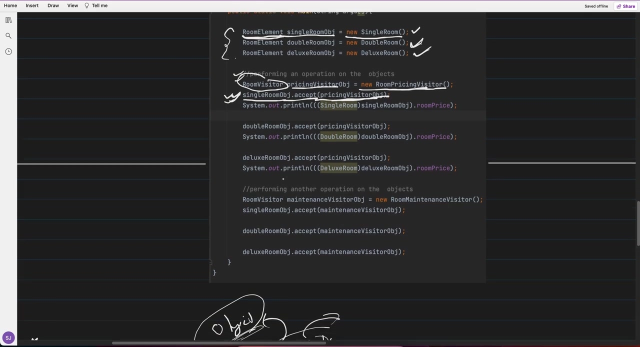 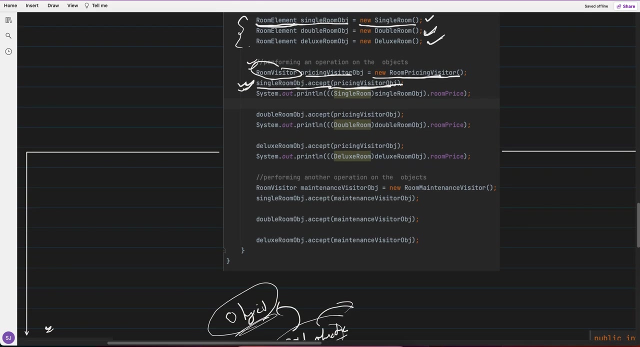 visit method. it has to call this visitor- sorry, not this one- this, this, this object, single room object right which we are invoking single room object. Now let's say i want to invoke the double room for the double room, i want to invoke the maintenance, so i have a double room object. this is the double room object right for the. 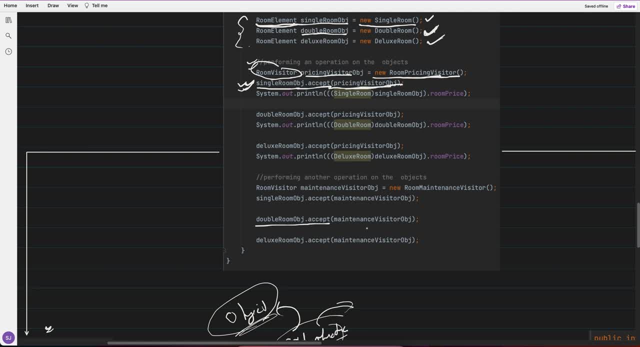 double room object. i can call except method. now i want to call the maintenance, so maintenance visitor. so because visitor is an operation, right, So maintenance visitor, operation Room maintenance visitor. i am passing. So first it will call the except method room element. so it's an interface, so this is a 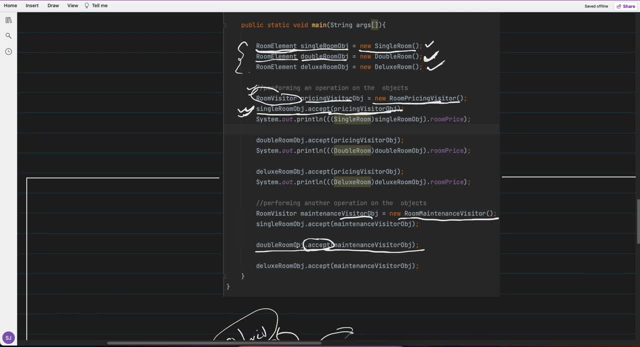 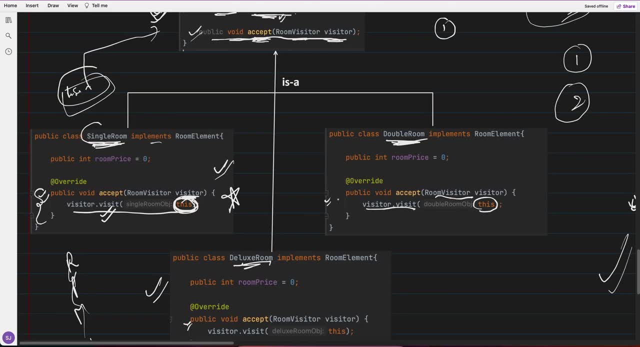 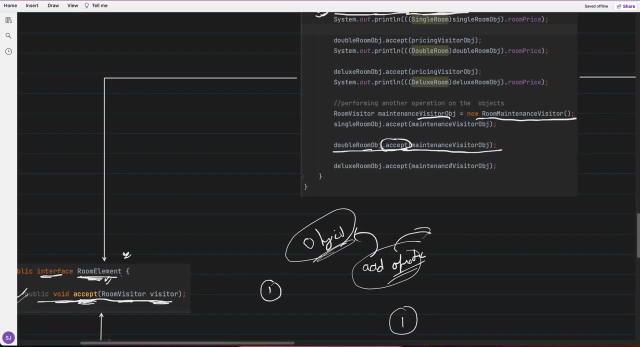 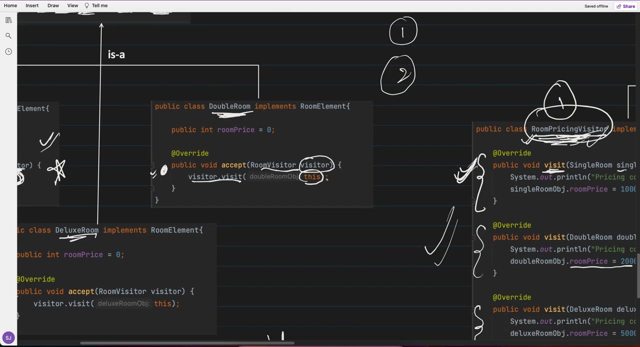 reference right. so it calls the except method of what double room? double room. so for the double room it will call the except method now. now, what is the visitor we are passing here? The first one we are passing is maintenance visitor objects. They are new room maintenance visitor. so what object? it will call room maintenance visitor. 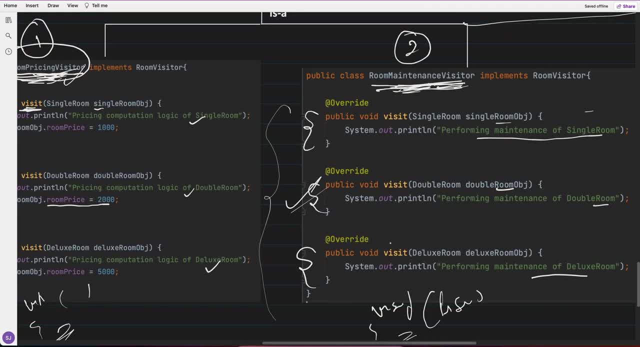 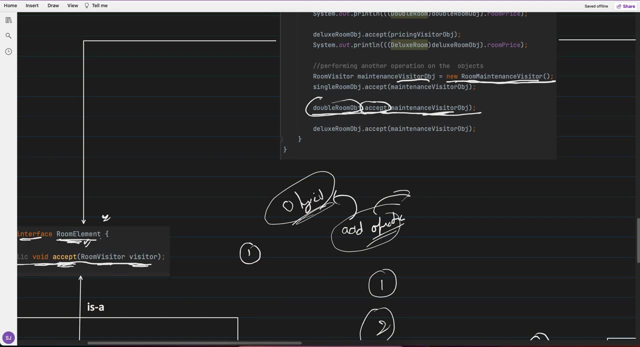 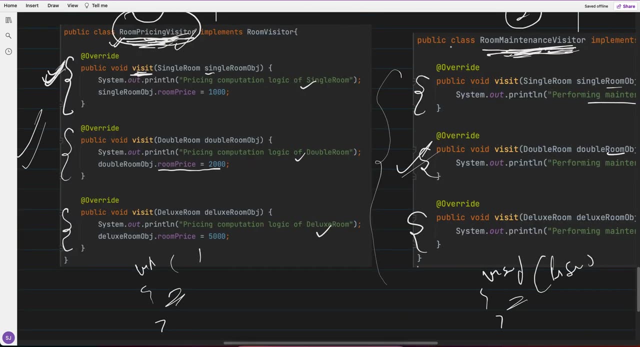 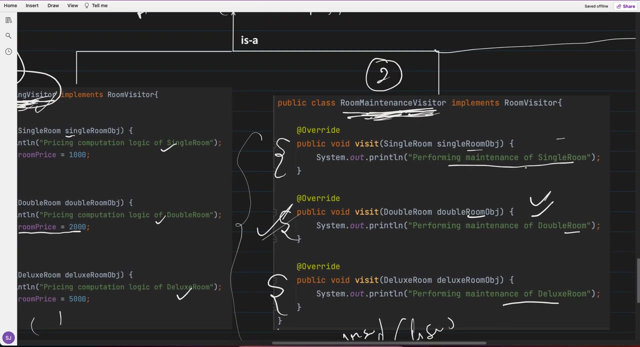 dot visit. So here, room maintenance with a dot visit now which offered it will call this: what is this one we are passing? double room, or here? this is the object, right, so double room object. we are passing This is the double room object, so it will call this double room, right, so here. i think it's pretty much should be clear by now. 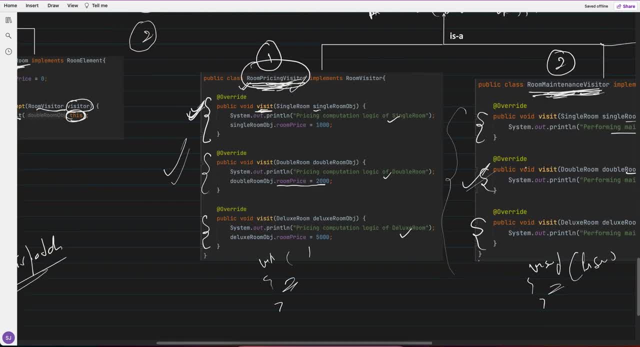 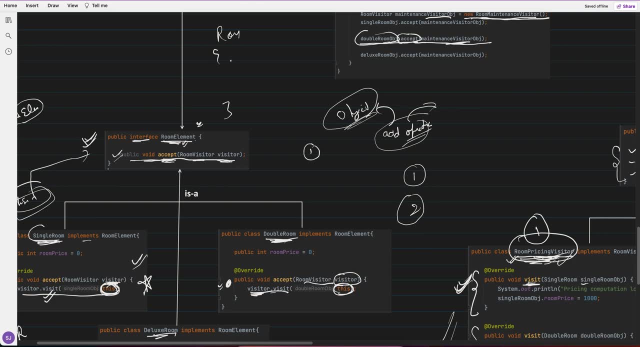 right what visitor is trying to do what, so it takes out of the operation from the class. earlier i used to have create room class and inside this room class i would have create reserve room, calculate price, do maintenance, all this thing. but now i have taken this method out. 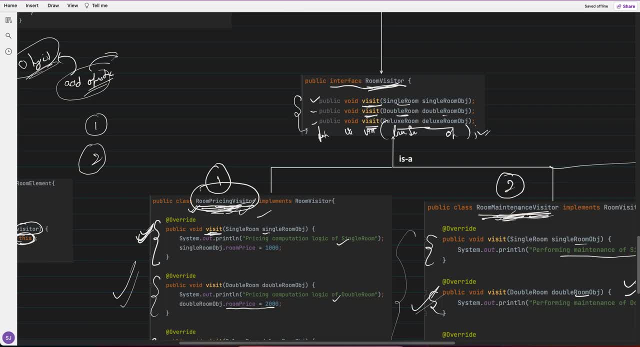 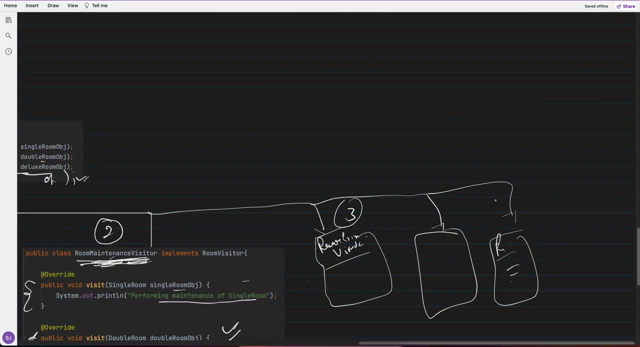 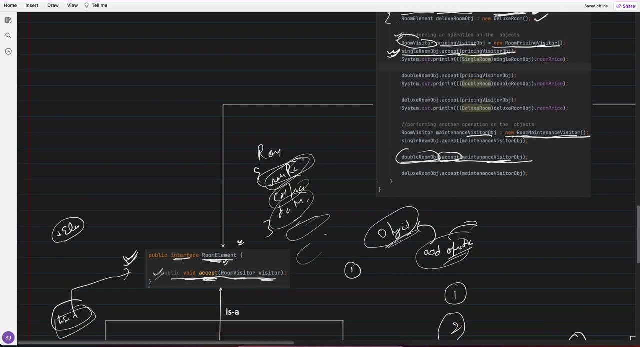 and for each operation i have created a visitor right and as soon as in future, more methods or more operation comes, i can add, keep on adding the visitor right and based on this, you already know that how to invoke a particular method. so that's actually while we are invoking right. we did double. 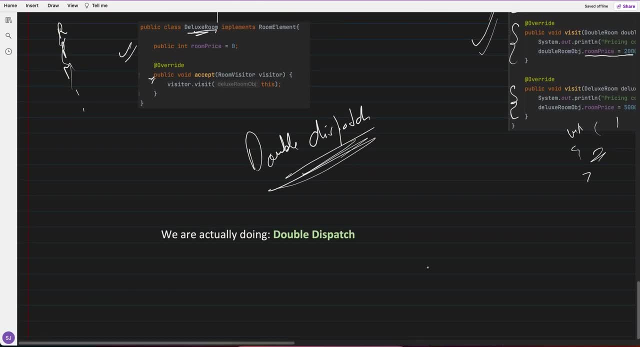 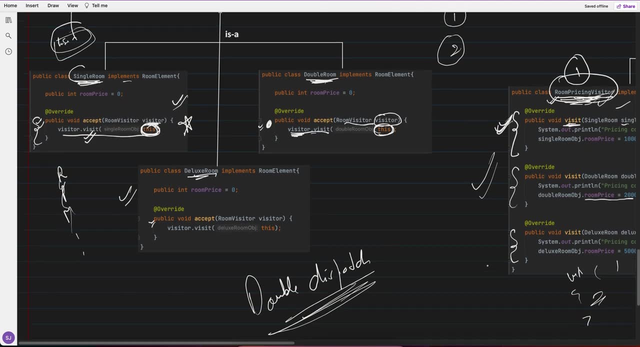 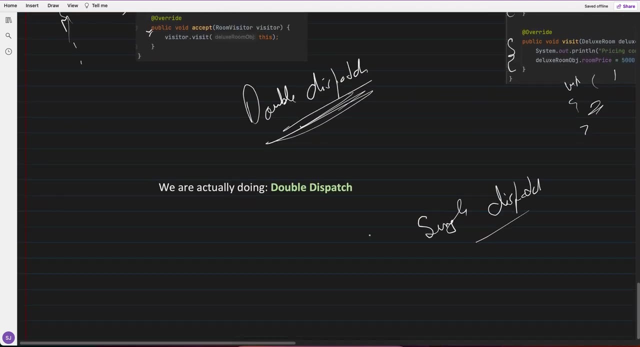 dispatch. so before understanding the double dispatch, you need to understand what is single dispatch. so see both. you already know we have done we what we have both we have done here: single dispatch, double dispatch here. but just to clarify separately that, okay, this is the single dispatch. so here, if 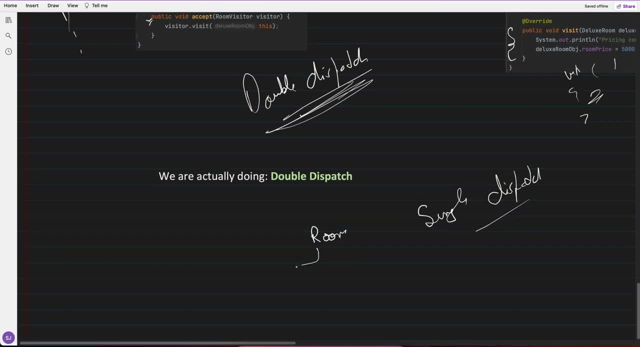 you see that we have a room, we have single room, double room, deluxe room, right, and it also has method except. it also has method except. it also has method except. okay, all three has method except. this is an interface. this is also has except, but it's an abstract. now, when you are creating an object like 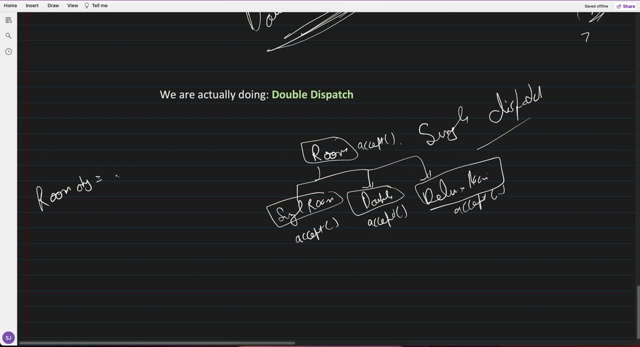 this room, obj equals to new deluxe room and you are calling objexcept. you know, right, it's a basic polymorphism, right? so with this reference, interface reference- you are calling an object or calling a method, but which method it will invoke, whether single room, double room or deluxe room, what so it will check. okay, this reference holds an object of. 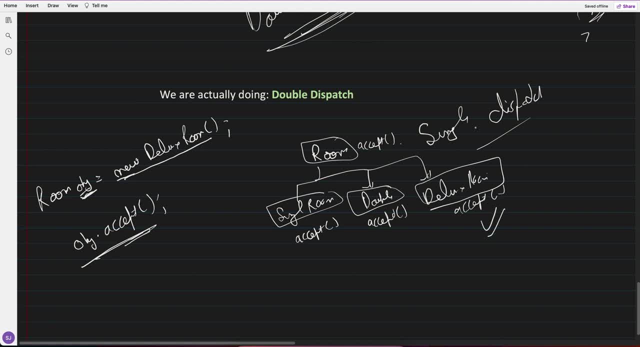 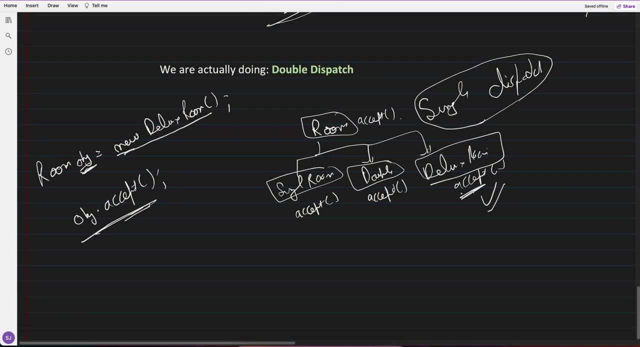 what deluxe room. so it will call this object. this is known as single dispatch. single dispatch means the method which has to be invoked. it's depend upon one object, right? so this method except which math except method has to be invoked. it depend upon one object, this: what object reference I hold? 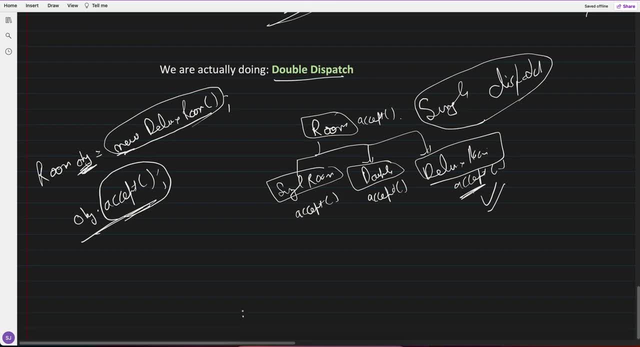 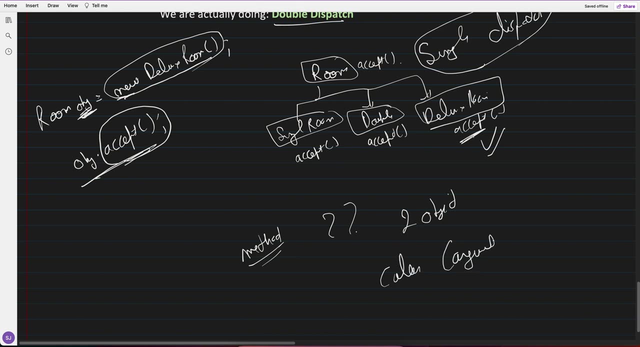 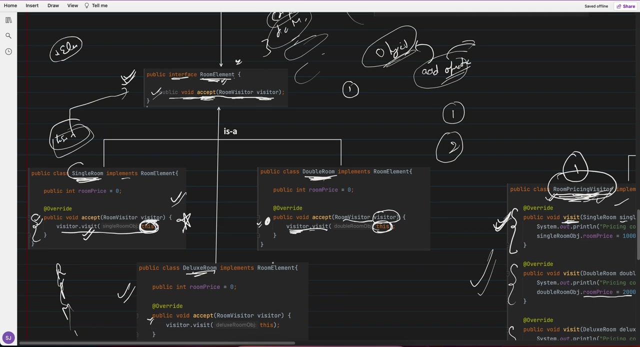 double dispatch means the method which has to be invoked. it depend upon two objects, right. one is the caller and another is argument. one is caller and another is argument. that is known as double dispatch. so here if you see that we are doing double dispatch here. so I'll tell you this. 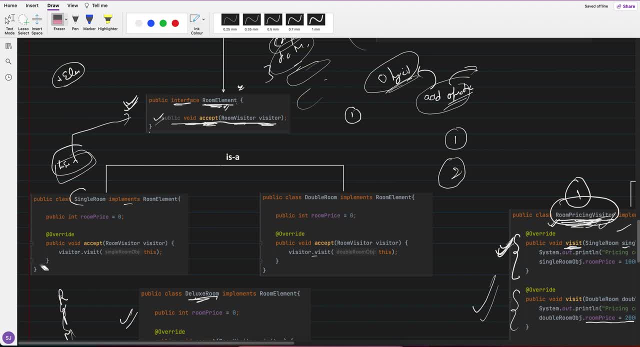 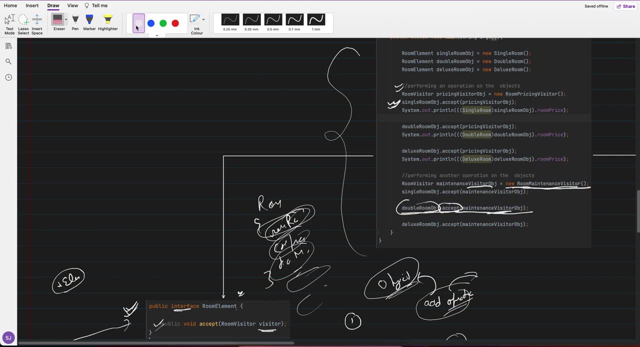 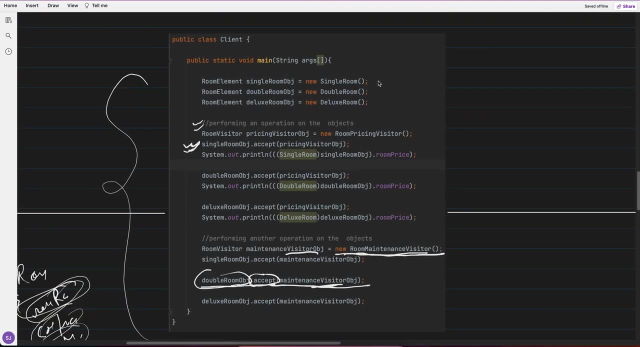 part where we are doing a double dispatching. so just little bit clear me up so that it would be. yeah, so let's see that double dispatcher so you can tell the force dispels it. so now I'm calling this method. just see this method. right, I am calling single room object, dot. except so single room object. this is a room. 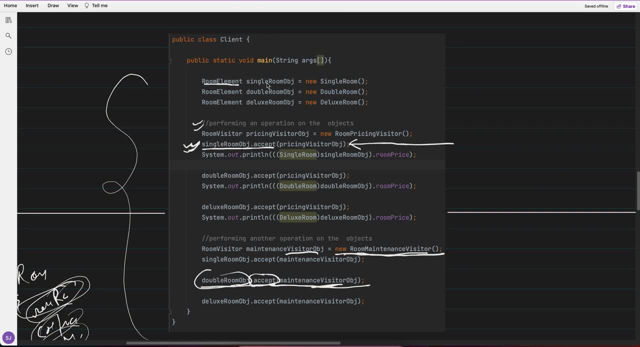 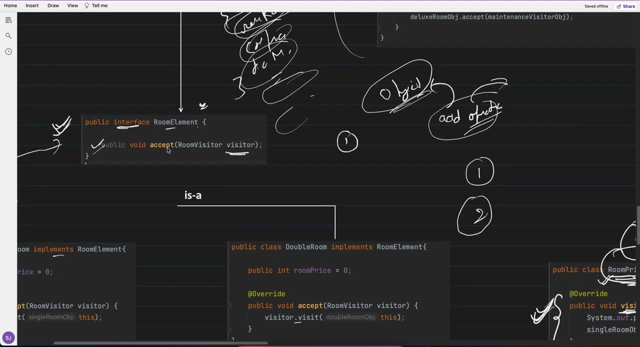 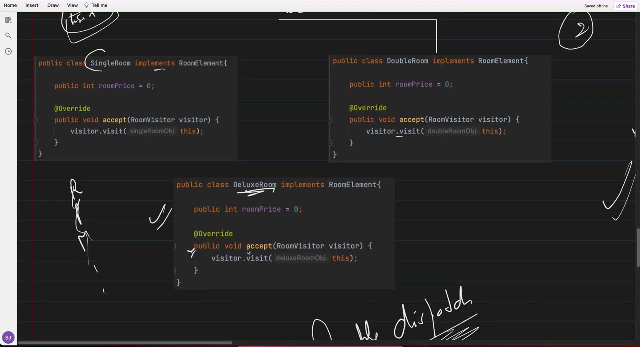 element: interface reference. this is just a reference. now it is calling except room element. this is element. we are trying to invoke an accept method and this is a difference. which accept method? it will call whether a single room, whether double room or deluxe room. it we will see that it's a 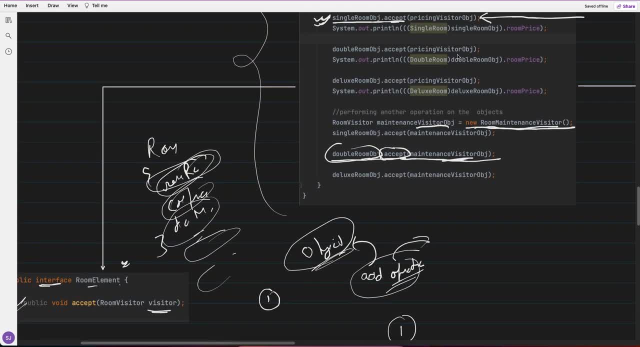 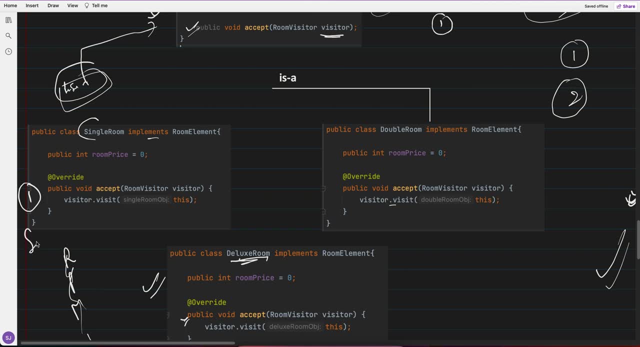 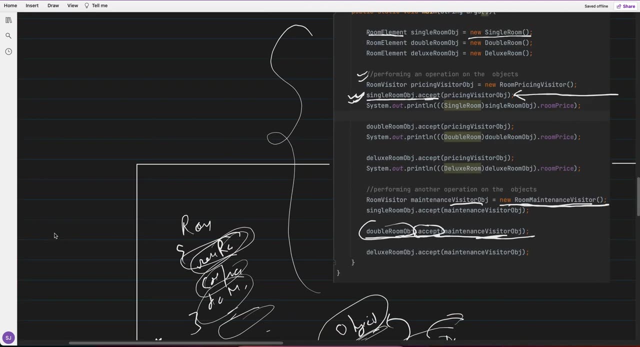 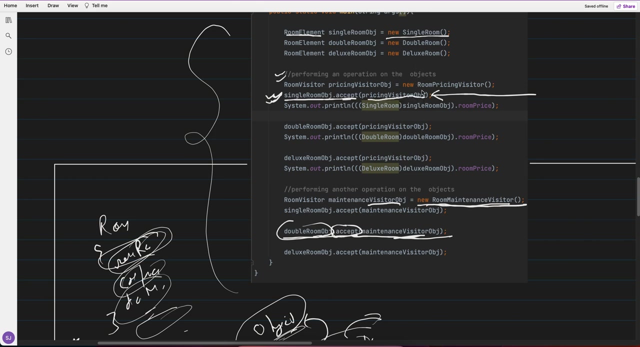 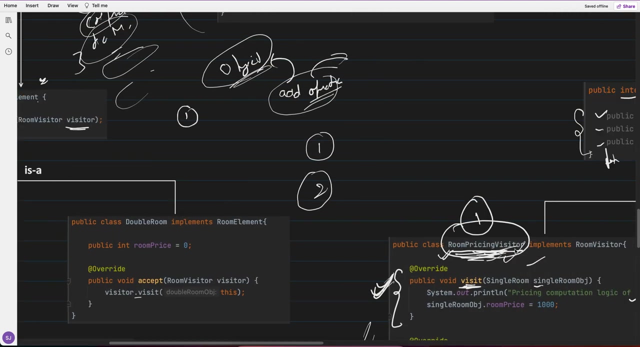 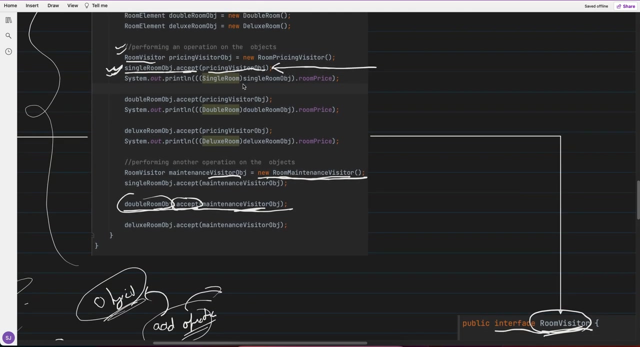 reference of single room. so which it will invoke this first. so this, what happened is single dispatch happen. this is single dispatch happen. now, here i am passing in the argument another reference, another reference, room pricing visitor. so here again, this is an room visitor, is an interface room visitor. here is an interface and i am passing this interface here reference. 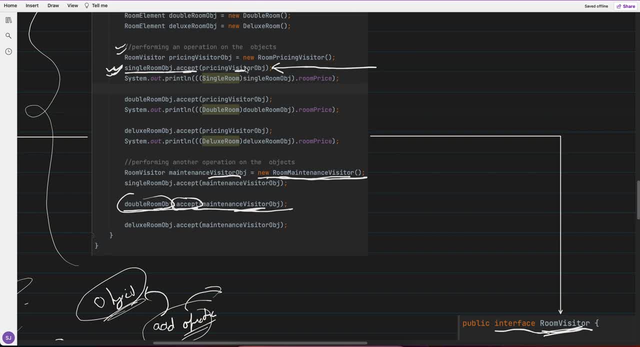 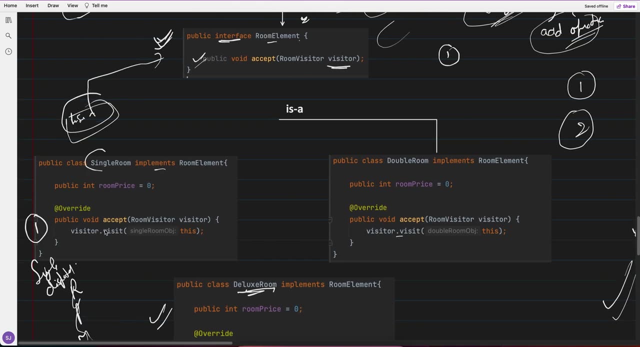 so i am passing this reference here. i am passing this reference here, but this reference holds an object. of what this reference object reference points to which object: room pricing visitor. so now here, if you see that when this accept method got invoked using single dispatch, this visitor was room pricing visitor. so now it is calling dot visit. now the second dispatch happen. 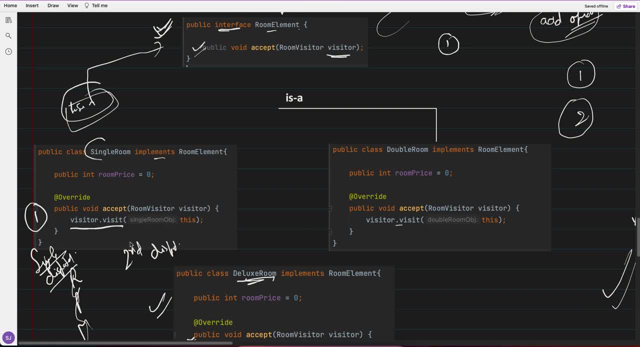 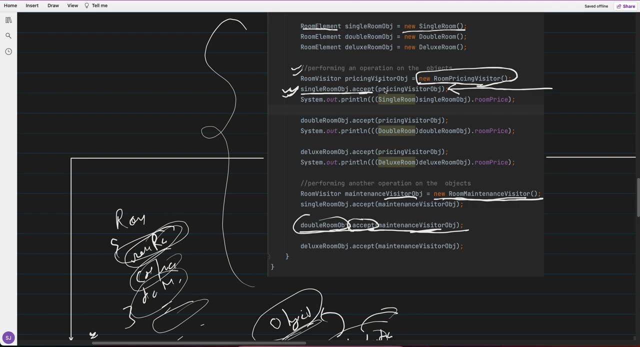 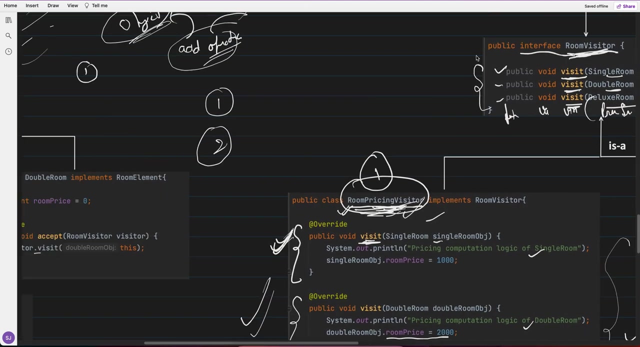 right. so here, if you see that this is the, actually the double dispatch is happening at this point of time. so this is the reference is happening. i am passing the reference here. right, room pricing visitor: right, but what element room visitor? the interface, now interface. i am calling dot visit. 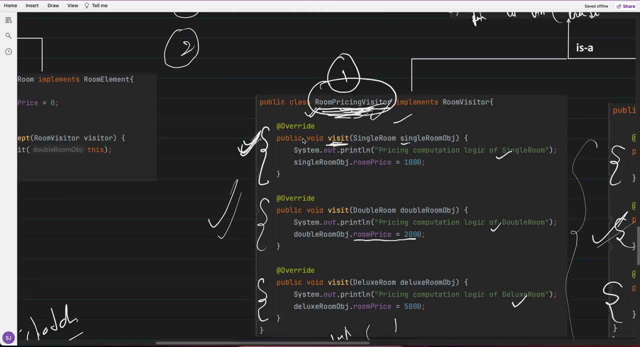 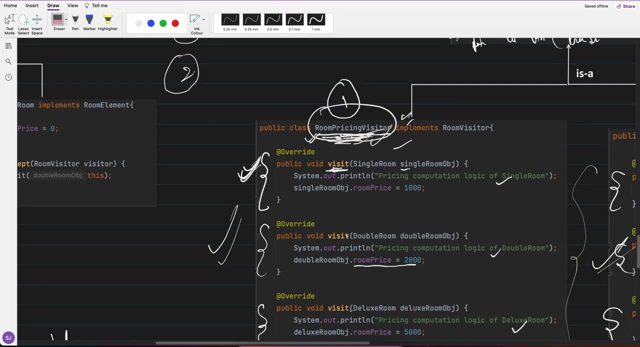 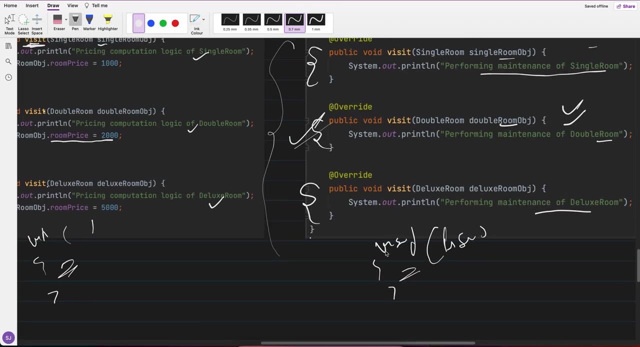 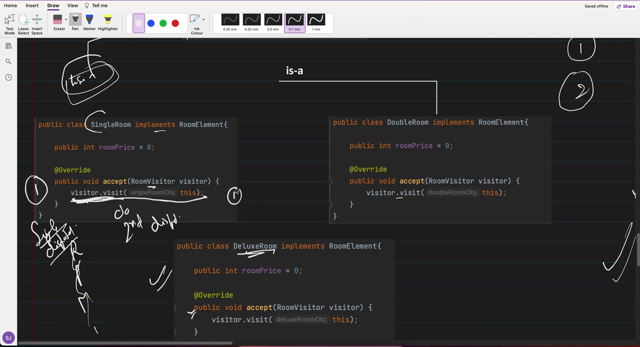 so there are visit, uh, so many visit, visit one, visit two, visit three into this visitor. then we have uh visitor and visitor here also in maintenance, visitor also. so which visitor i am talking about? so it does a first dispatch here, first dispatch is single dispatch, it does, is, is. 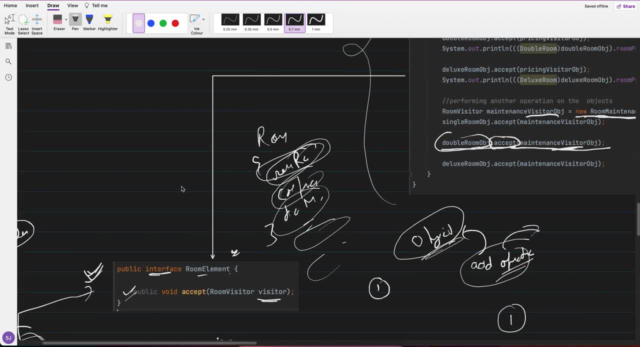 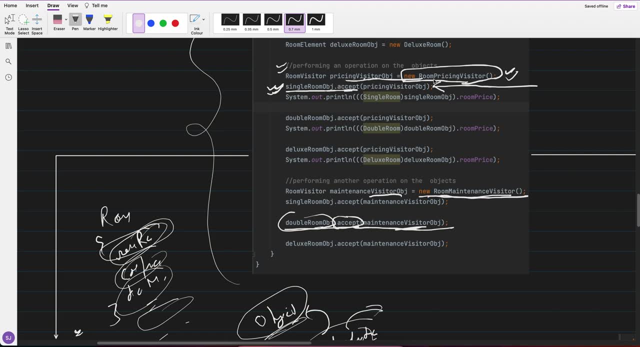 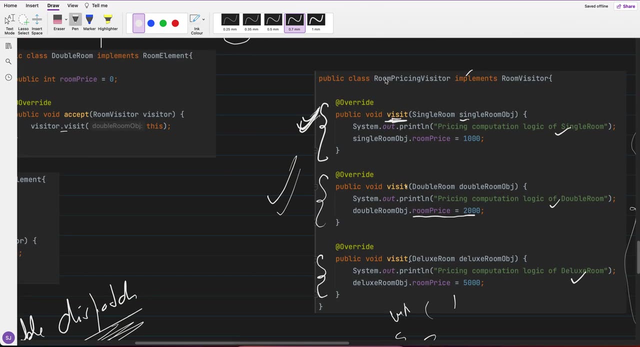 this room visitor is pointing to what? so internally it will calculate. okay, this, it is triangle. this reference is pointing to this room visitor, room pricing visitor. okay, so it knows that. okay, it has to call the visit method of this room pricing visitor first, first dispatch happened, now double dispatch. 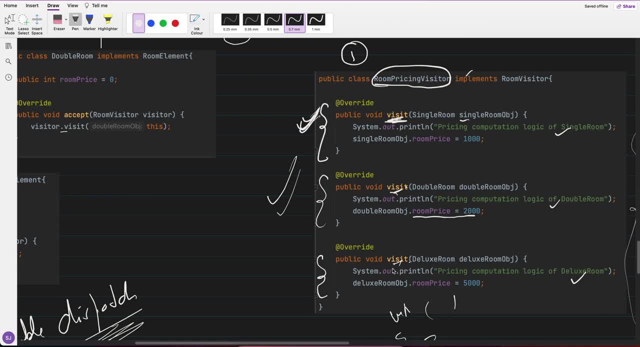 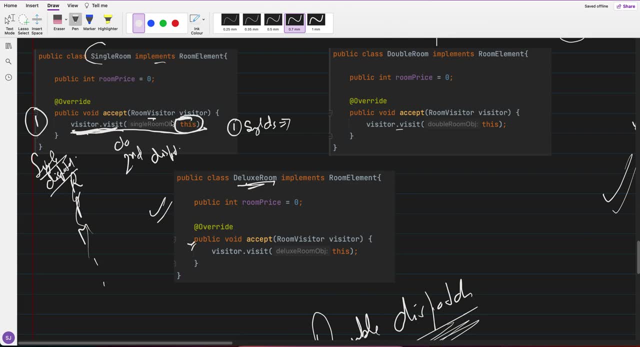 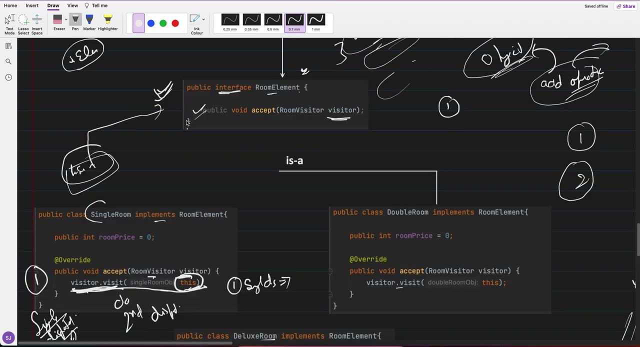 okay, this class also has so many visit, visit, visit. now, which visit to call? you are calling visit control, but which visit now? this is the second parameter. this is the second parameter. so now it is telling that, hey, this object. so what is the object it is passing here? single room. object: single room. 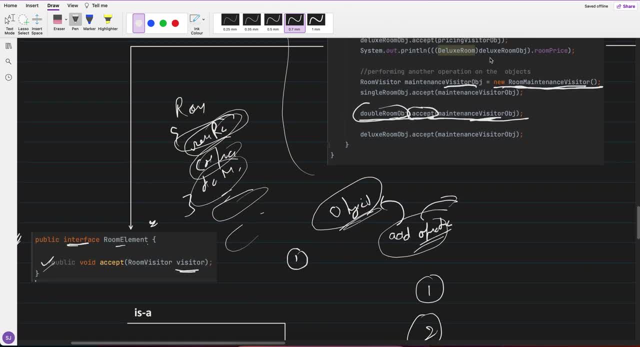 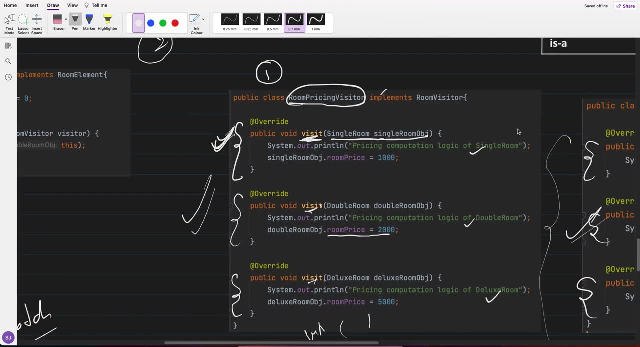 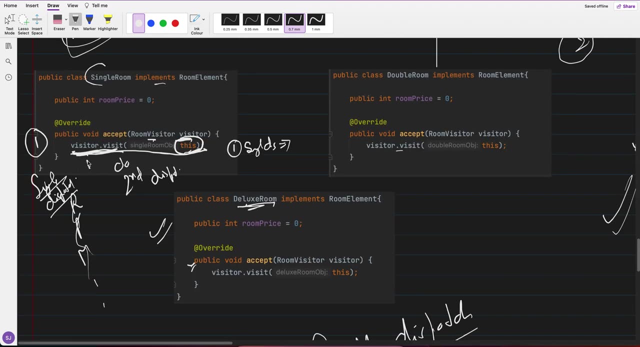 object, again pointing to the new single room. so it will call new this single room. so now here. if you see that the method which has to be invoked is now dependent on two objects, first the caller and the second the argument with the caller- you get to know that. okay, this is the class. 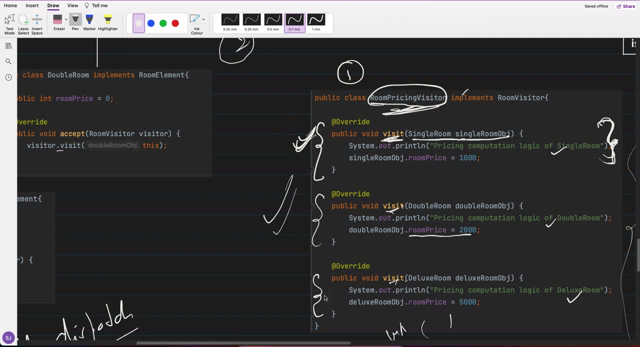 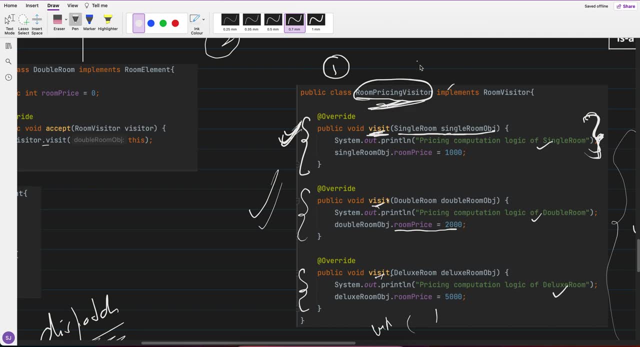 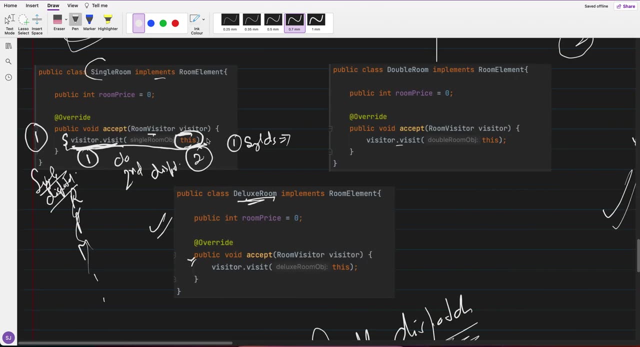 in which this visit method is exist, because there might be different classes in which the visit method is there. okay, so with the first caller, you got to know that, okay, this is the class through which, in which the visit method exists, but if there are more than visit method which visit this, this reference, which hold this reference, so this is. 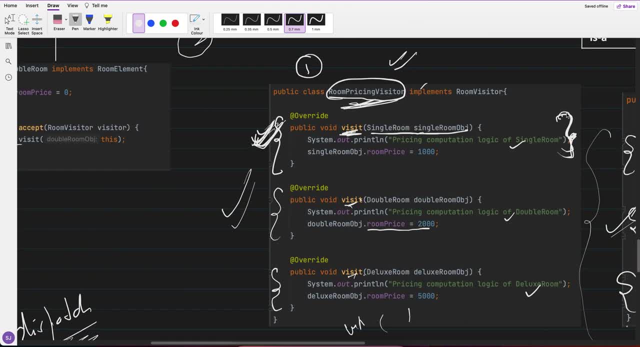 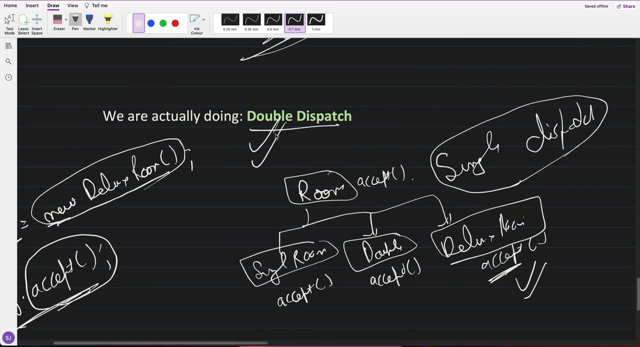 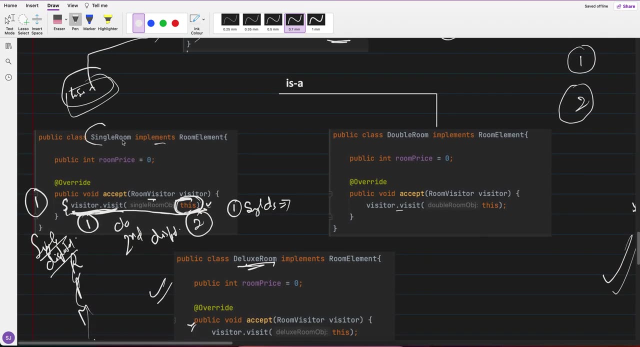 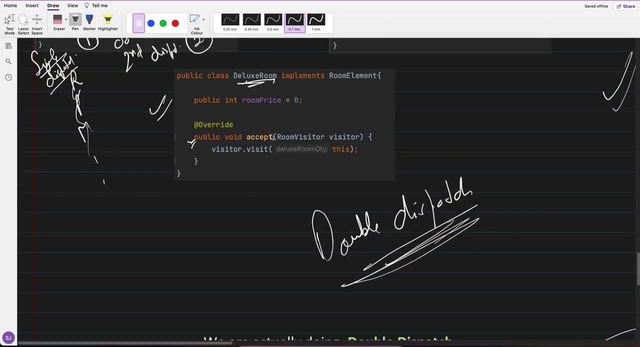 the single room object reference right, so this one. so the method is decided based upon the caller and the argument. so visitor pattern uses double dispatch functionality to take out of the operation from the object or element. i hope this is should be pretty much clear, like what is the? 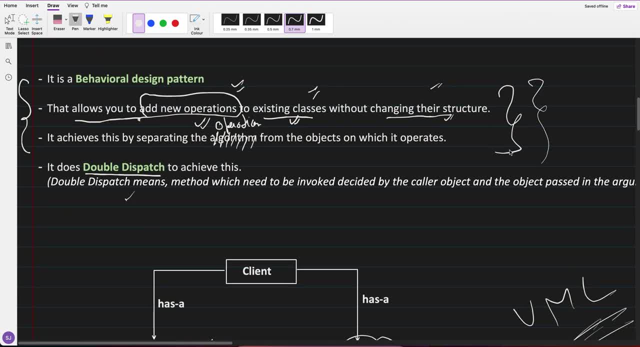 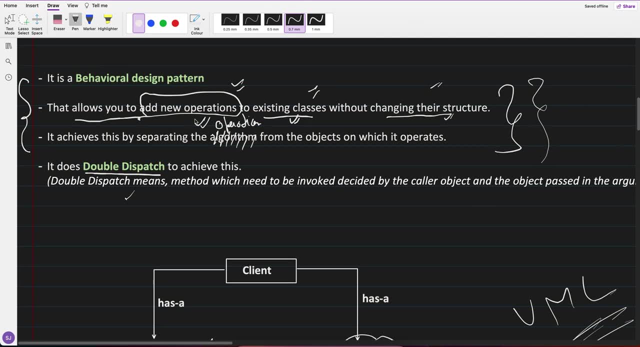 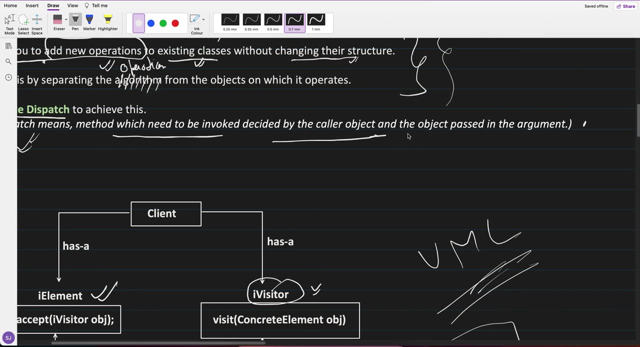 problem. what is definition actually allow you to add new operation without changing the existing class? how it is you? what is double dispatch? double dispatch mean method which need to be decided by the caller object and the object passed in the operation argument. so i think this, i think it should be clear, with an example itself. so at what? 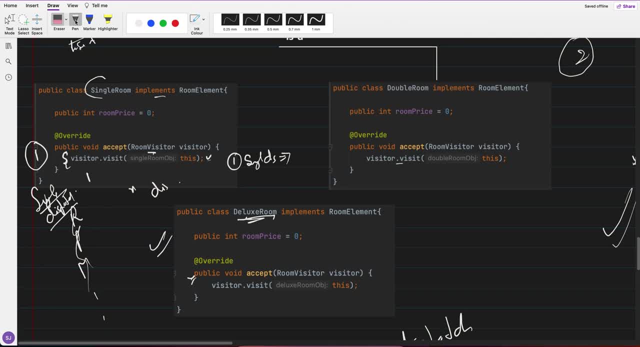 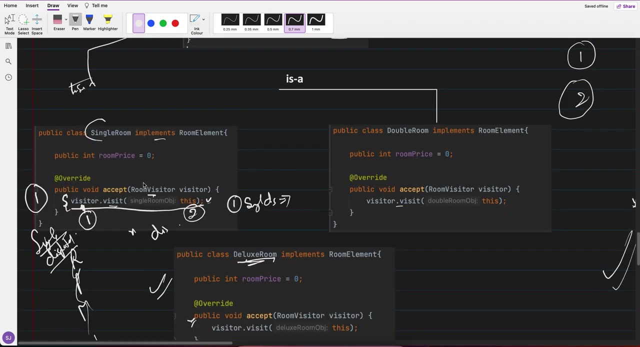 time double dispatch is happening. this, this is actually. we are doing double dispatch. first, this is the caller, first it will determine which class and if that class has so many visit a particular visit method has to invoke, then this argument will help: which particular method? okay, and single dispatch. i have already told you that single dispatch is nothing but. 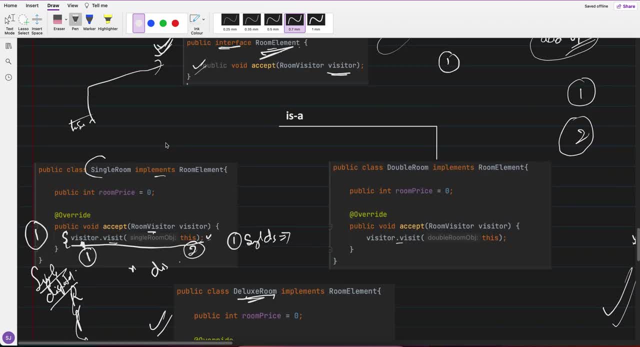 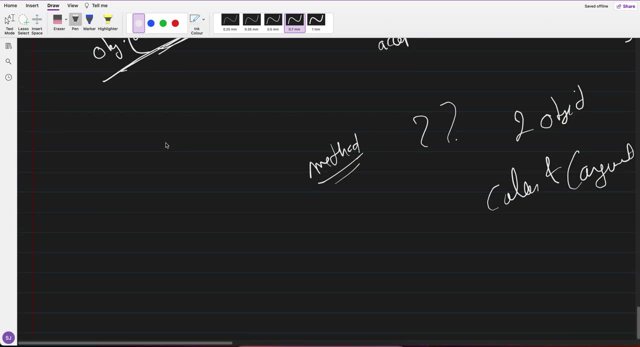 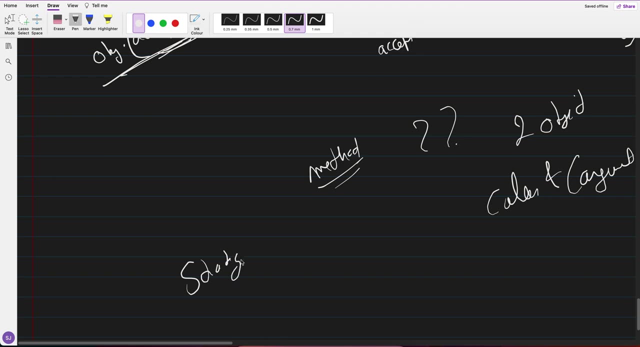 a normal polymorphism with a simple example, right. so this is the visitor pattern here. and before going, if you stay till here, then i will tell you like many people get confused it with the strategy design pattern, because in a strategy pattern, let's say, if you have 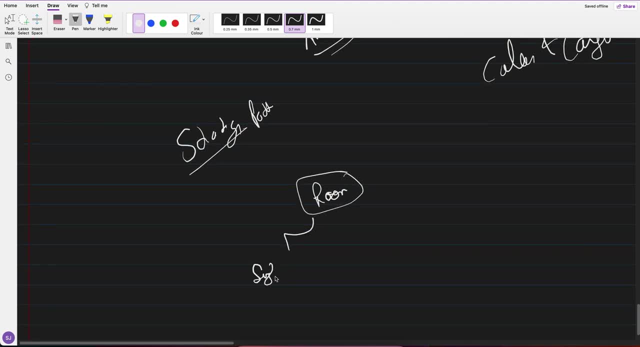 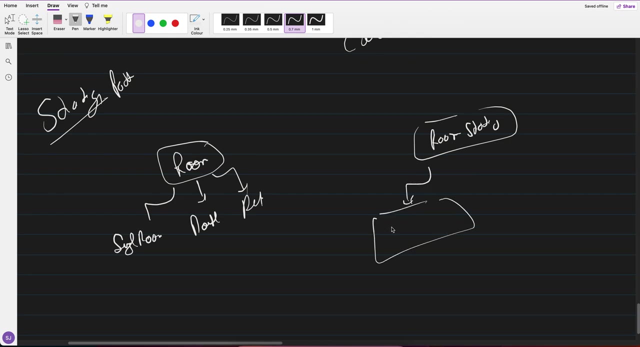 room. you can have, let's say, single room, double room, deluxe room, and then you can have, let's say, room strategy. what they will do is they will do room strategy and they will try to put it like this: hey, i can have a single room pricing strategy, i can have single room. 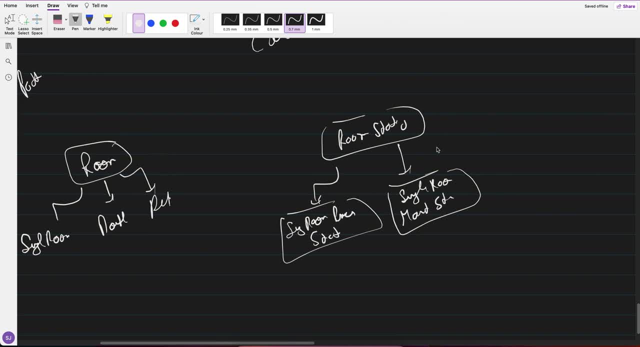 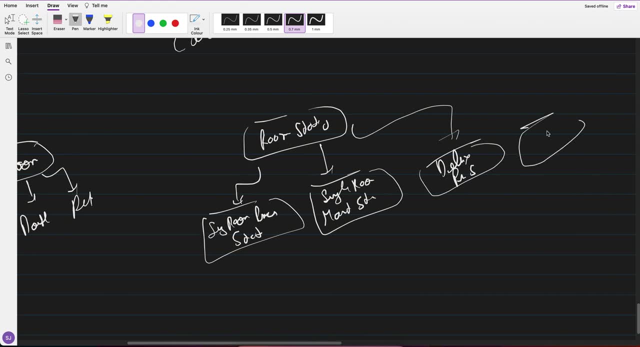 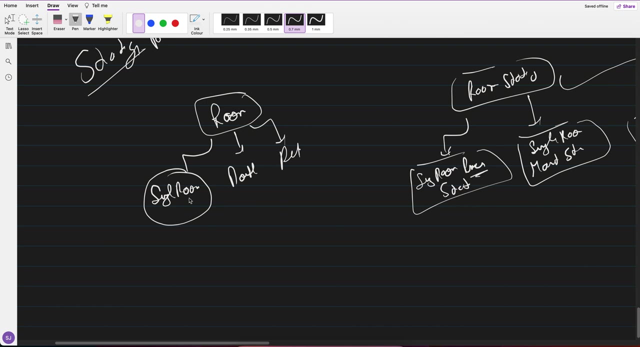 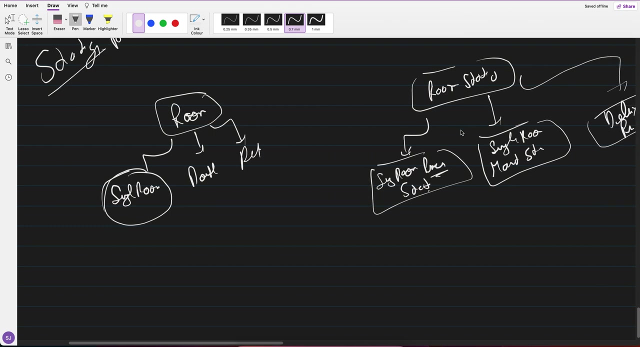 maintenance strategy like this. i have deluxe room pricing strategy, deluxe room maintenance strategy and now, whichever strategy i have to- let's say, i want to use pricing- single room pricing- i can dynamically runtime pass this strategy and i can use it. no, yes, you can do that, but this is wrong. 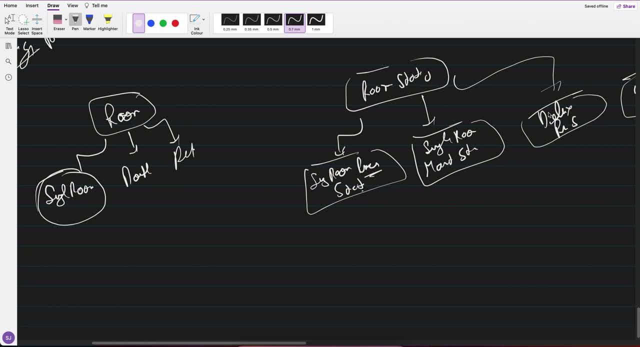 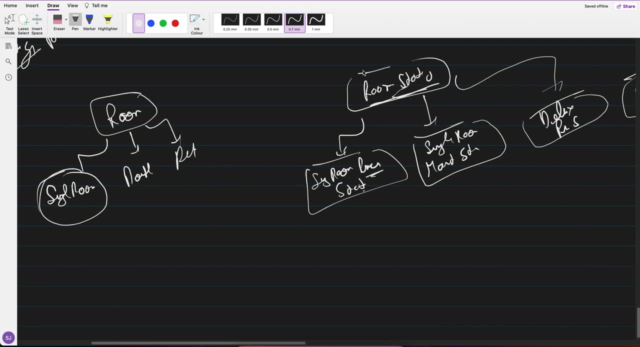 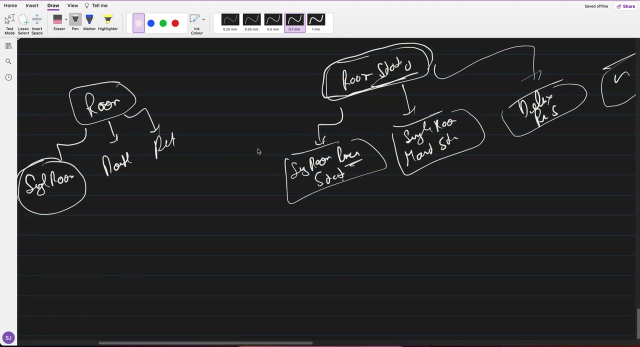 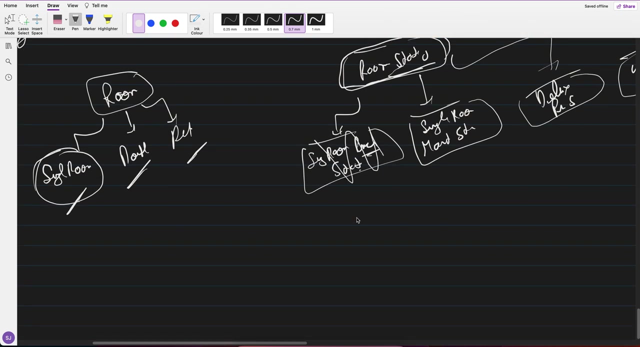 see, these are all operations. strategy pattern is mostly for separating out the algorithm. right, that's why i have cut it at above. it's not algorithm, it's operation. so strategy pattern separates out the algorithm. algorithm is independent of this, elements like single room, double room, so algorithm can be like, let's say, if it is like this, price calculation algo.